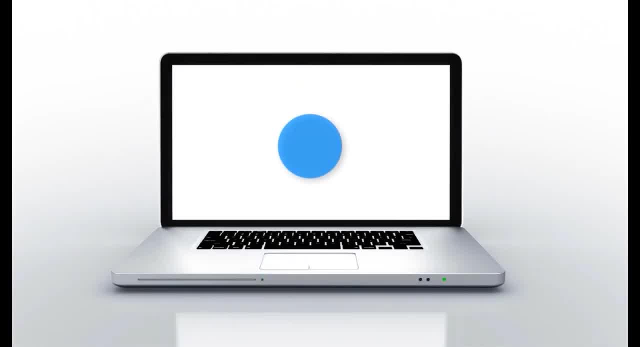 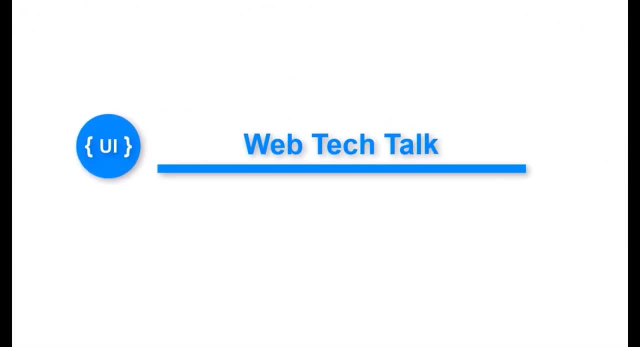 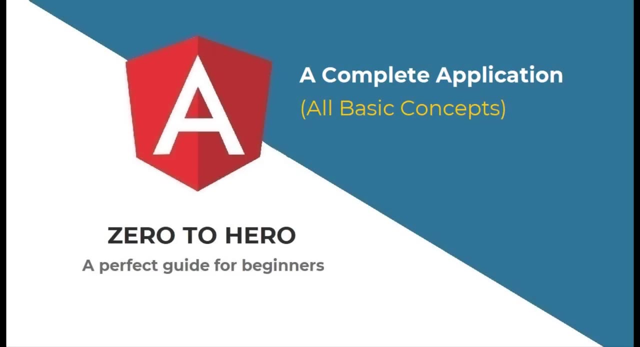 Hi friends, welcome back to the brand new series on Angular 0 to Hero- a perfect Angular guide for beginners. In my last video I have explained about how we can use pipes in Angular to transform the data, And with that we have completed all the basic concepts in Angular. 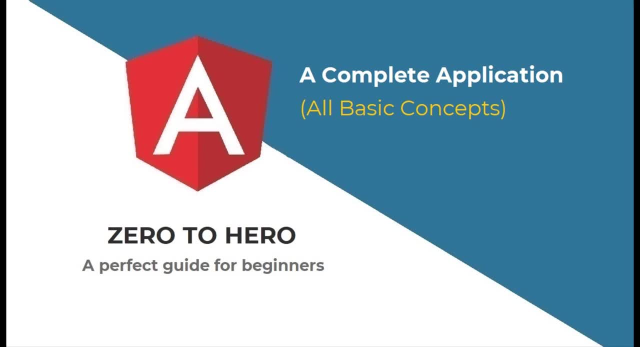 Before we close this Angular 0 to Hero series, let's create a simple Angular application or a final project in which let's try to use all the concepts we have learned so far. Let's start. Okay, let me show you the final application which I am going to develop: Rotten Potatoes. 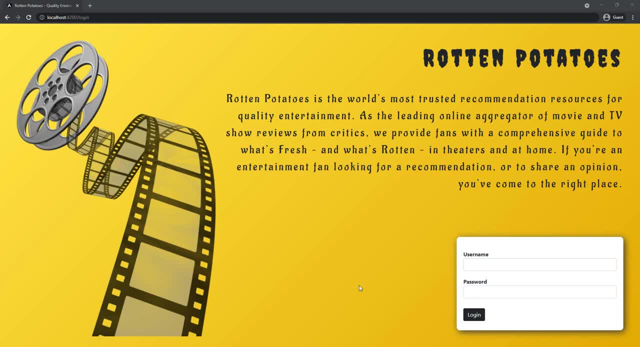 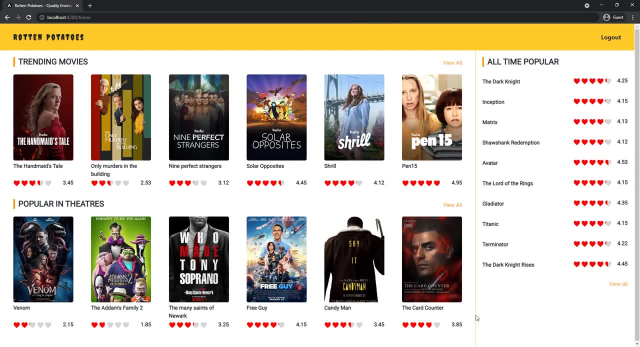 The name seems to be funny Here. I have a login form to enter username and password. When the user enters the right username and password, user will be taken to the landing page. Here in the landing page we can see a list of trending movies, a section for popular. 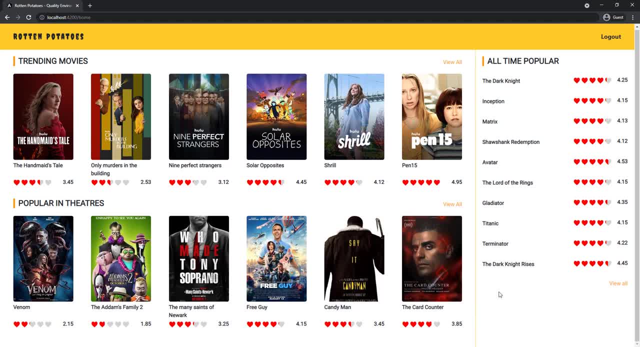 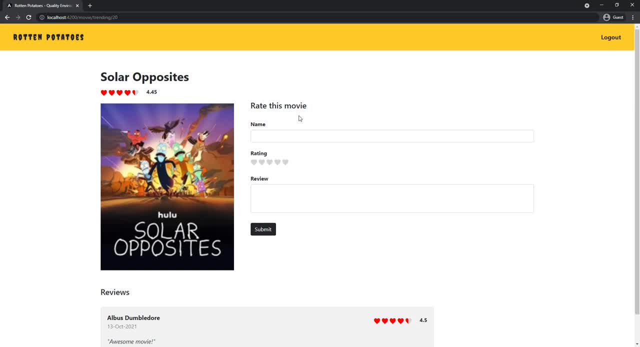 movies running in theaters and all-time popular movies in the right. All have ratings available and user can click any of the movies to see the detail about the movie reviews and also the user can rate the movie using a form. Finally, the user can also log on. That's. 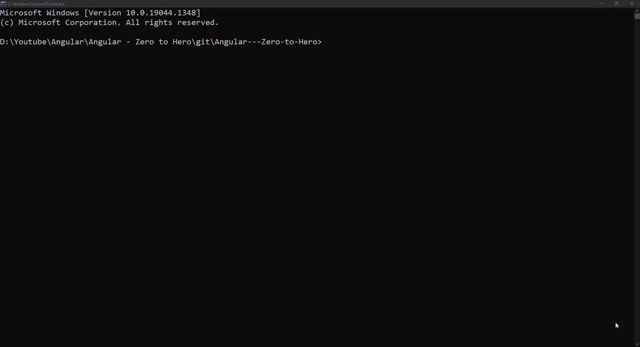 it. Okay, let's start. First, let me create a new Angular application ng new application name. Okay, it is asking me whether to enable stricter type checking, Let me choose S. And then it is asking whether I need routing- Definitely S. And finally it is asking me: 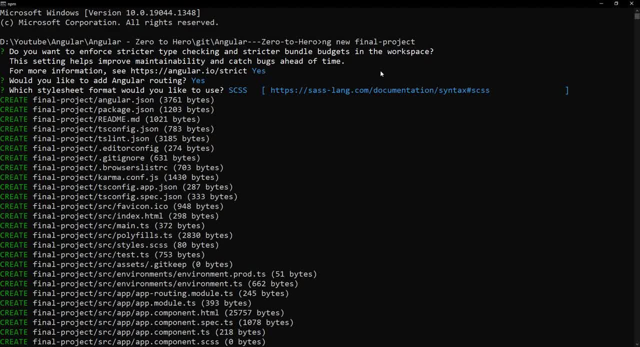 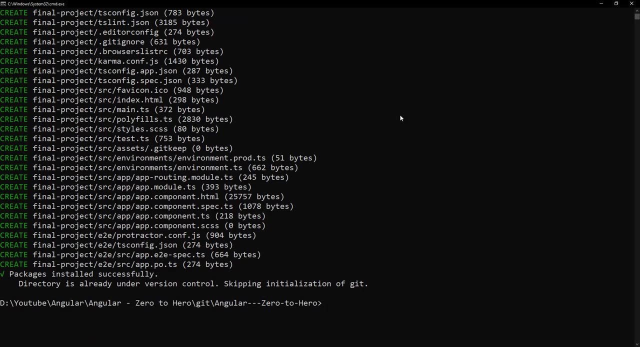 to choose the CSS format. Let me choose SCSS. Hope you remember the advantages of choosing SCSS over CSS. The application is getting created. This little amount of time depends on our computer speed. Okay, the application is created. Let me get into the application folder. Now let me install. 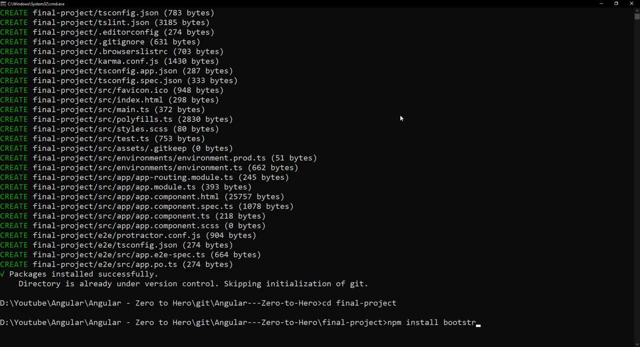 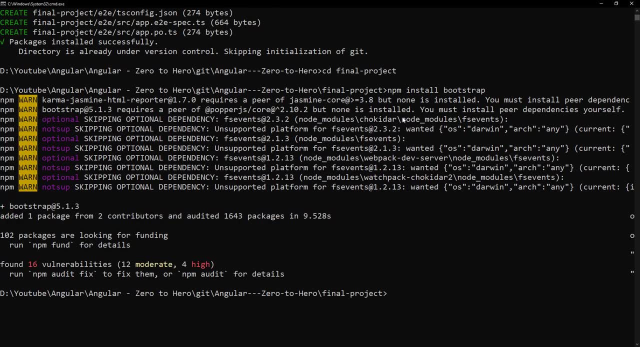 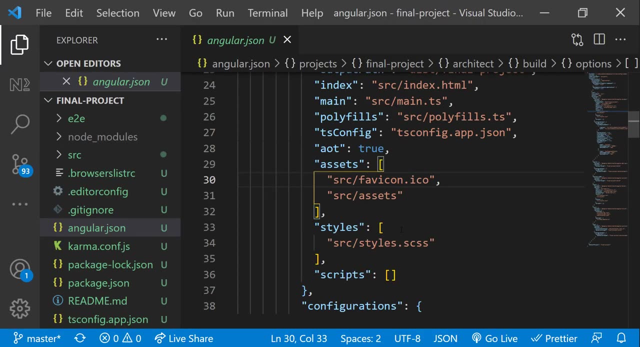 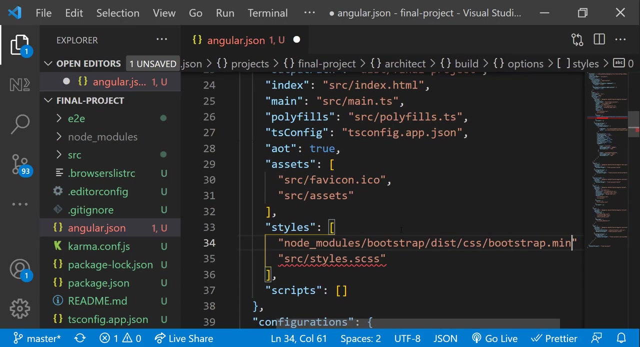 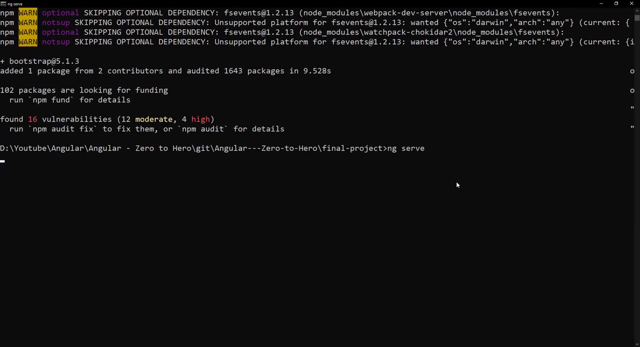 bootstrap- npm- install bootstrap. Okay, bootstrap is installed. Now let me open this code in VS code and configure bootstrap in the angularjson. Let me start the server: ng-serve. The server is getting started First time. it takes little. 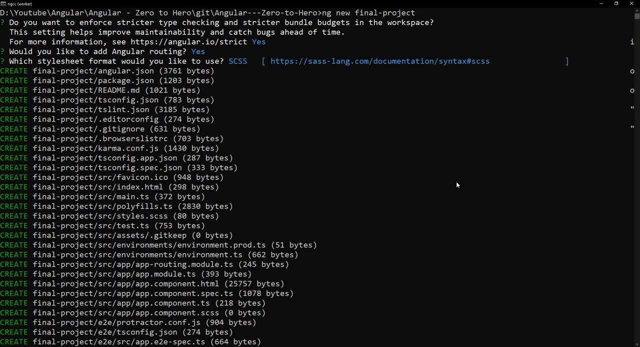 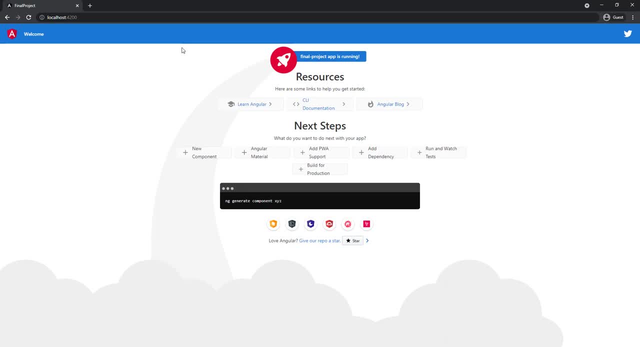 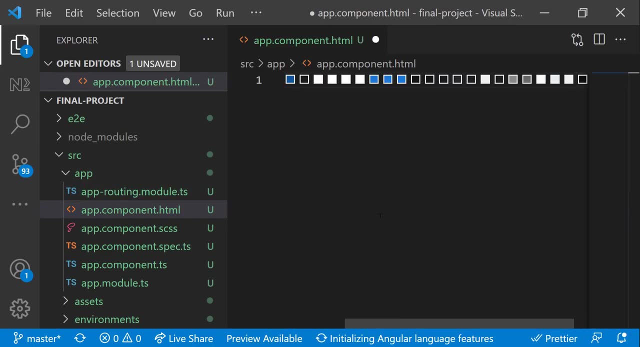 time to compile everything. From next time onwards, it will start quickly. Okay, the application has started. Let me open the application And if I delete the existing code and add a button with any bootstrap class. 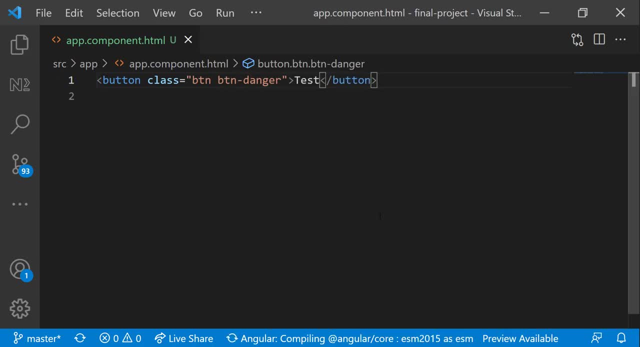 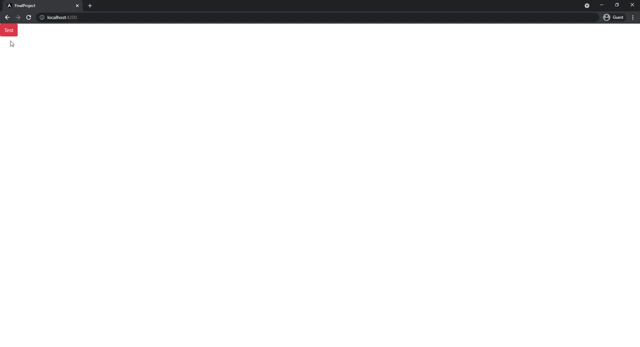 I can make sure the bootstrap is installed and configured correctly. First I need to create the components needed for this application. I need a login page, and then I need a home page. I can keep a common header, and so I need to create a header component. 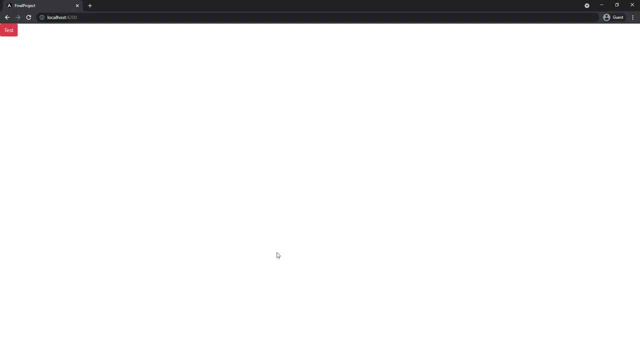 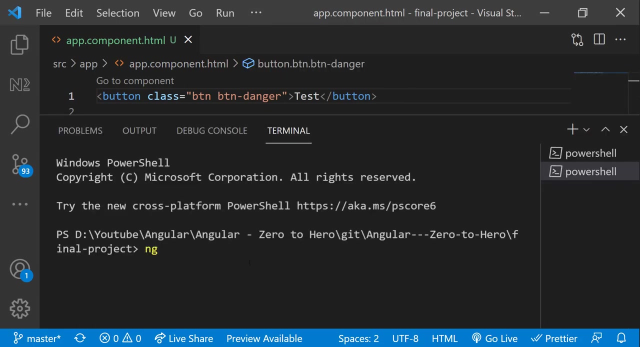 and finally, I need to create a component for detail page. Let me name that component as movie. So first let me open the terminal in the VS Code To create a component. I can use ng generate component component name: login Login component has been created. 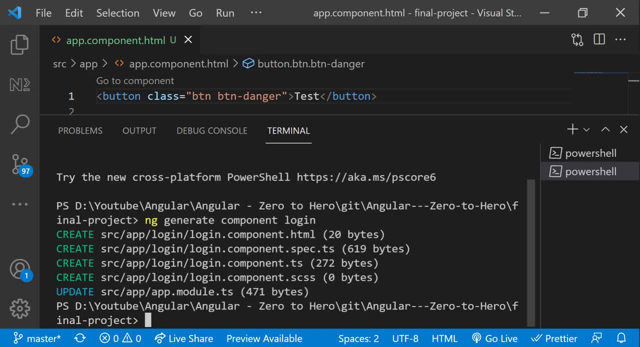 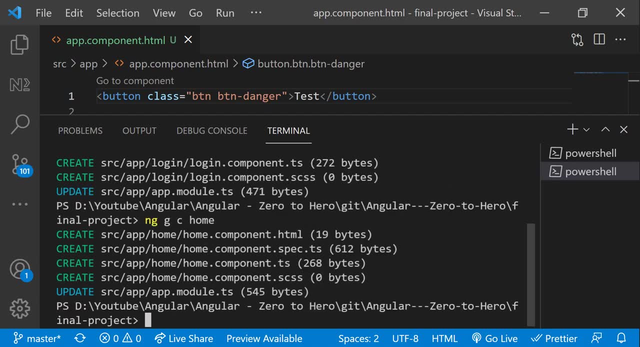 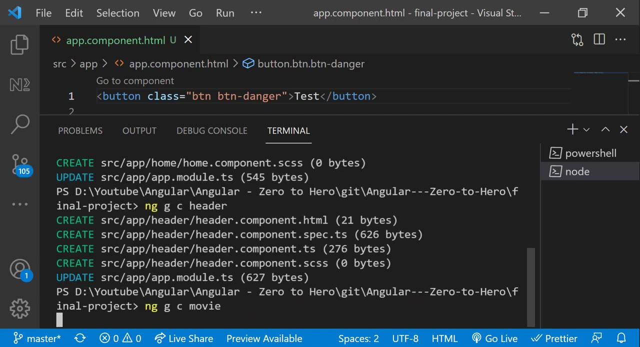 Now let me create the home component. I am going to use the shortcut command now: ng g c- home. Let me also create the header and the movie component. That's it for now. If I need any more component, I can create it whenever needed. 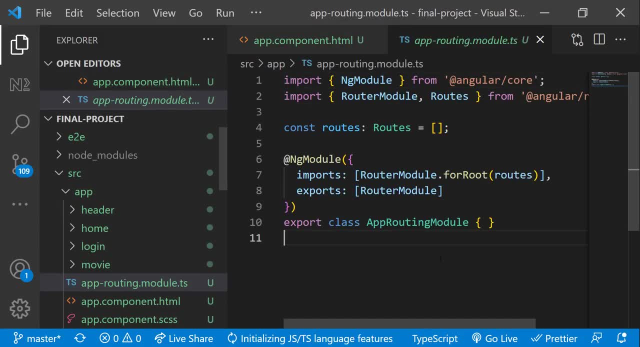 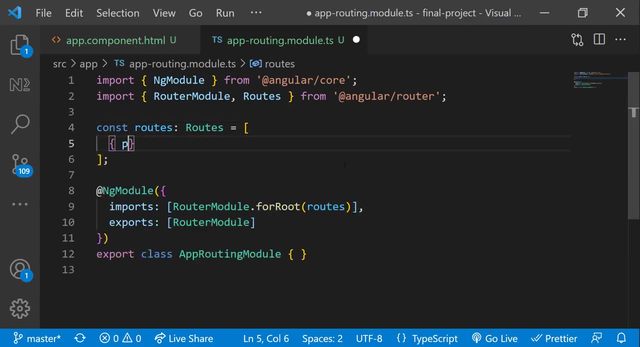 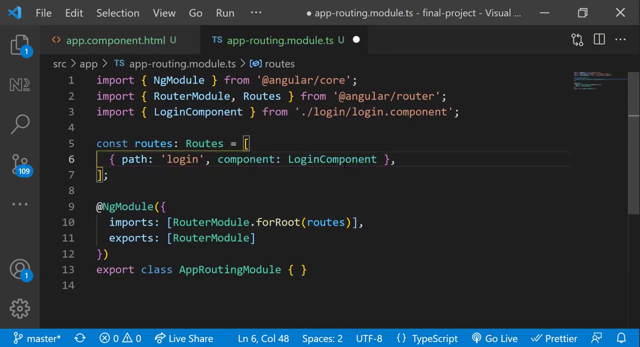 Next, let me configure our routing. I am opening the app routing module. Right now the routes array is empty, So inside the routes array, let me add the routes. When the path is login, I need to open login component. And when the path is home, let me open home component. 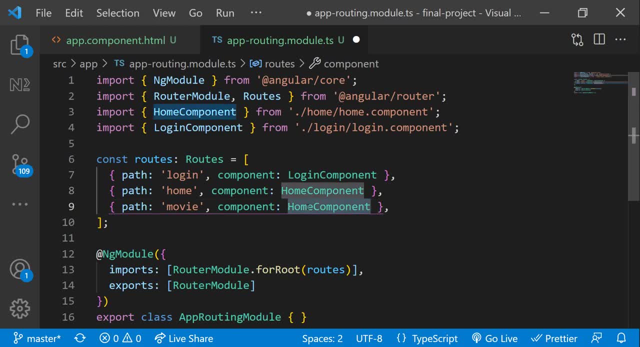 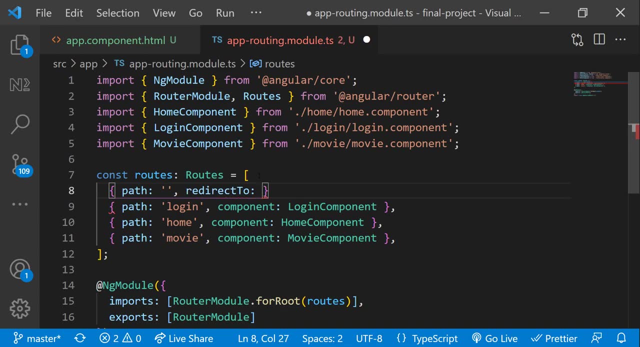 When the path is movie, I can open our movie component. And what should I do when there is no path? Let me redirect to the login route And make sure you add the path match when you use empty route with redirect to. And finally, let me also show the login page. 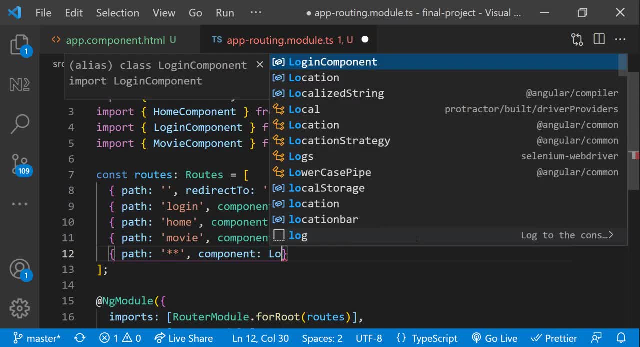 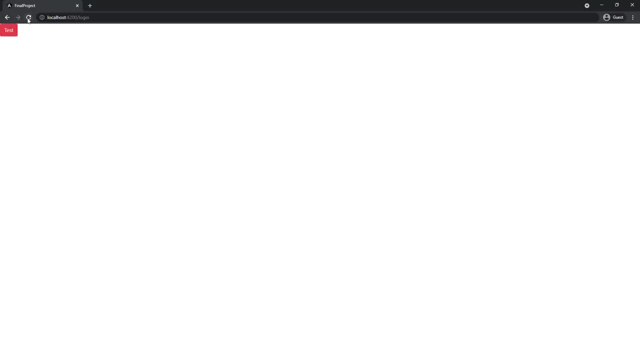 when none of the path matches using the wildcard route. Remember, it should be the last route always. Am I done with routing configuration? Let me see If I go and refresh the application. it is redirecting to login, But ideally I should see this one login works. 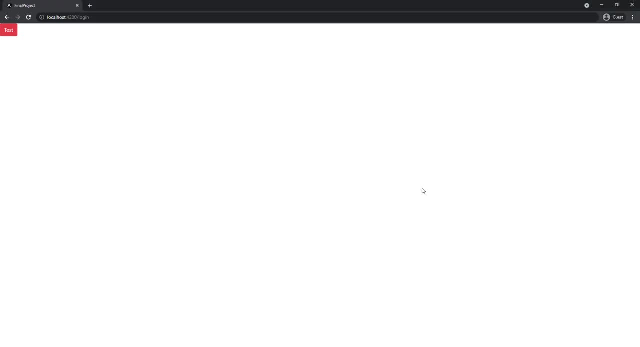 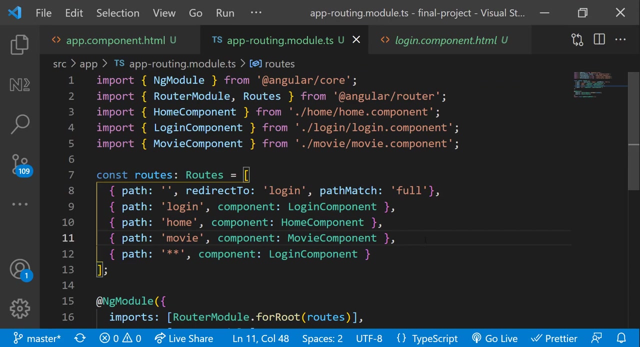 But I'm seeing the button. So what is wrong here? I have informed Angular what to do when it meets the route, But I haven't informed yet where to resolve the routes. So I need to add a router outlet. So let me go to the app component and add the router outlet. 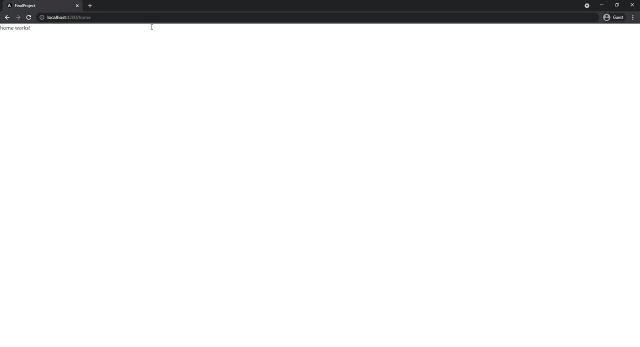 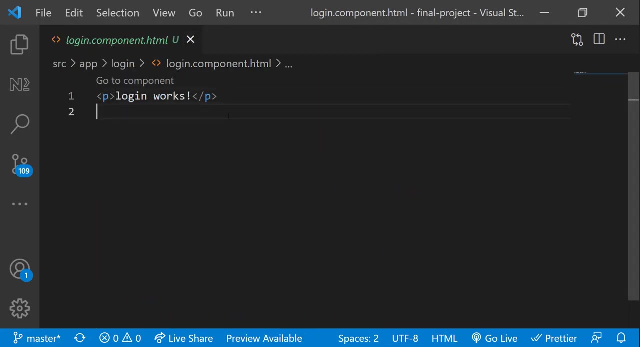 Now we can see login page is loaded correctly. If I change the route to home, we can see the home page is loaded. That means our routing is done. That means our routing is working as expected. Okay, let me start with the login page first. 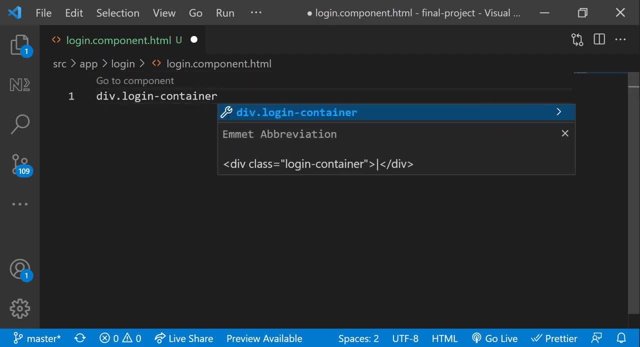 In the login component html, let me add a login container div And inside that I'm adding a logo div and a description div. Let me also add some contents. And then, in the login CSS for login container, let me give a width of 100% and a height of 100bh. 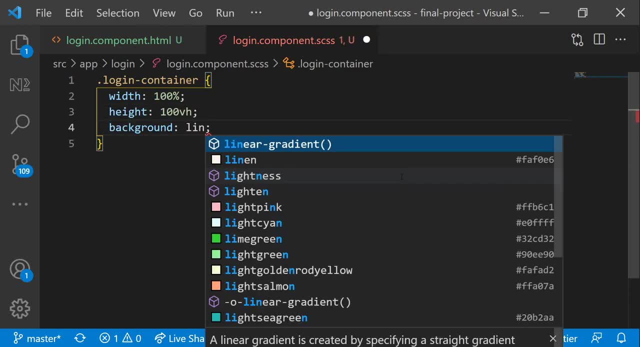 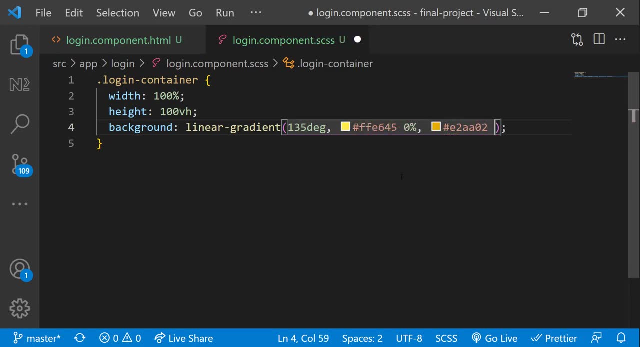 so that it occupies the entire screen, And let me also give a gradient yellow color background. Here is the preview. Okay, Now let me position the logo and description in the right side related to the login container. For logo, let me use a font size of 70 pixel. font-weight bold. 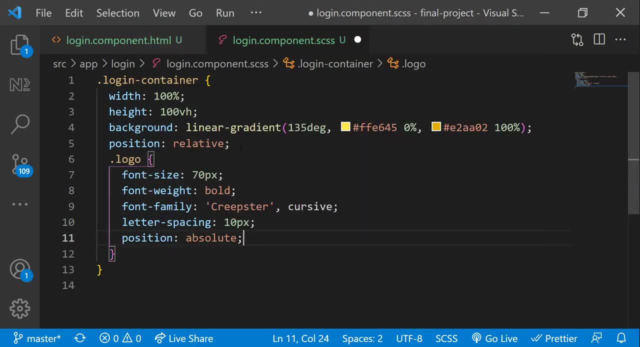 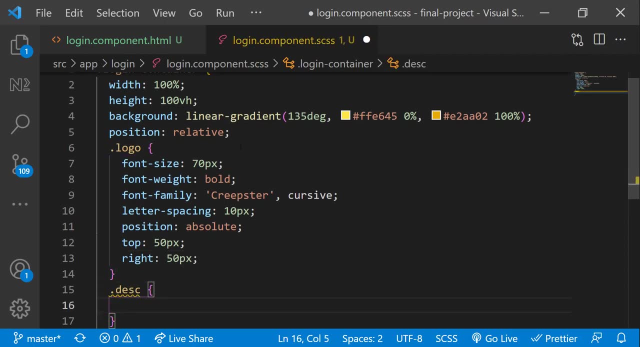 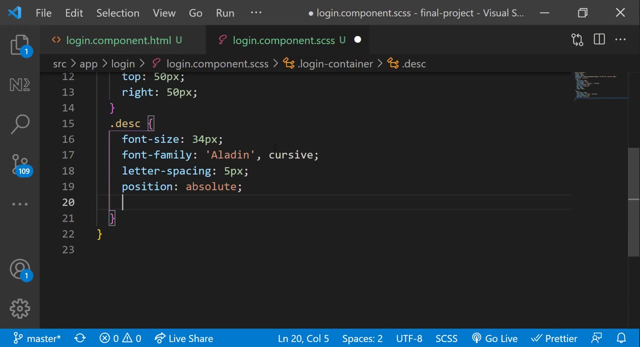 font-family creepster letter- spacing: 10 pixel position- absolute width- top 50 pixel And right 50 pixel, And for description I can use a font size of 34 pixel. font-family aladin letter- spacing- 5 pixel position- absolute width: top 200 pixel. right 50 pixel. 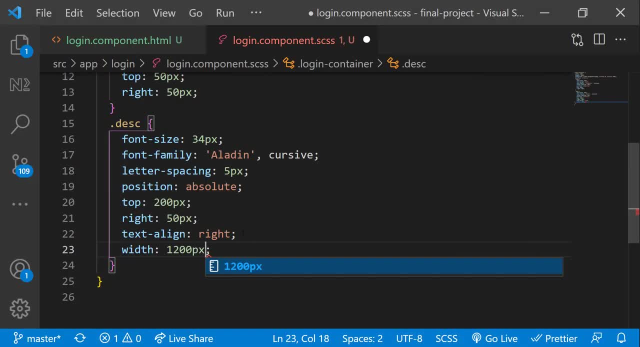 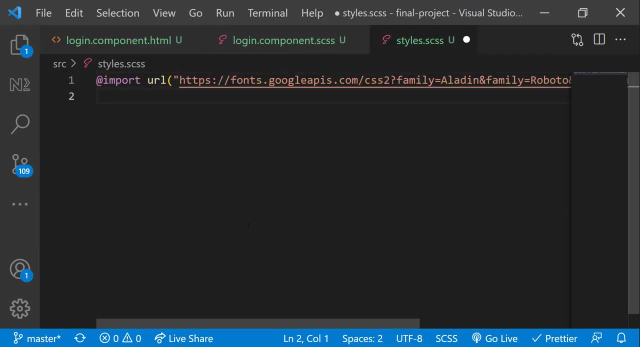 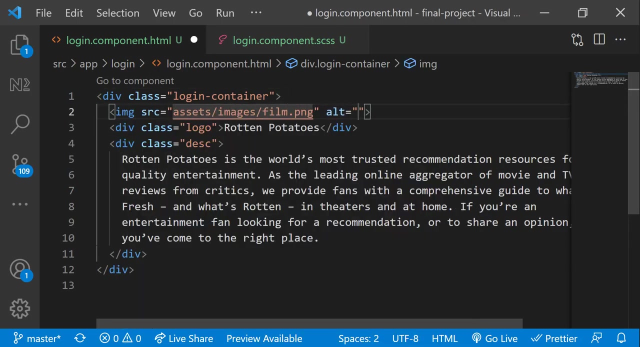 and text line right. Okay, it's too big. Let me add a width. Okay, let me also import the required fonts in the global styles. And I found one image. I'm going to add that to the assets folder and position that here. 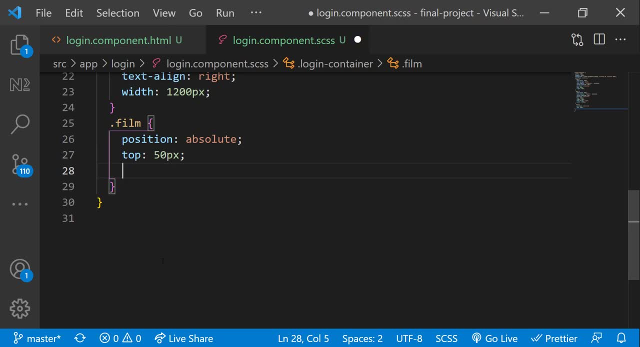 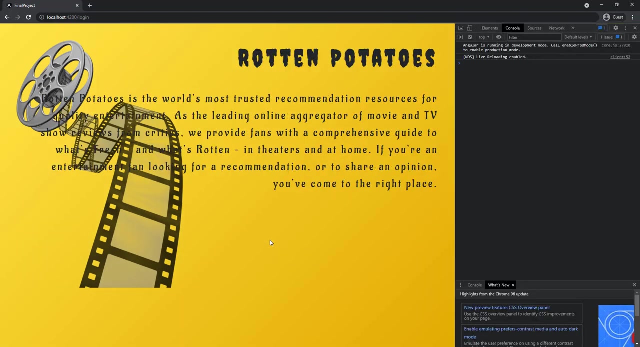 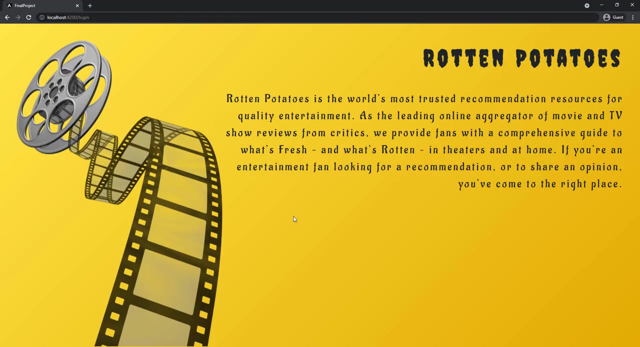 Let me give position: absolute: top 50 pixel and left 50 pixel. It is too big. Let me add a width of 500 pixel, Little small. now Let me inspect. Okay, let me add the login form. I have user name and password, so two form groups. 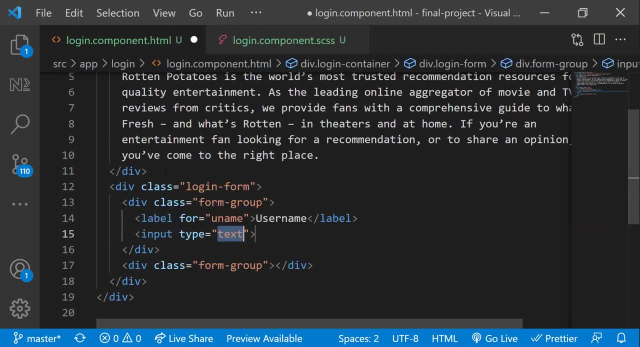 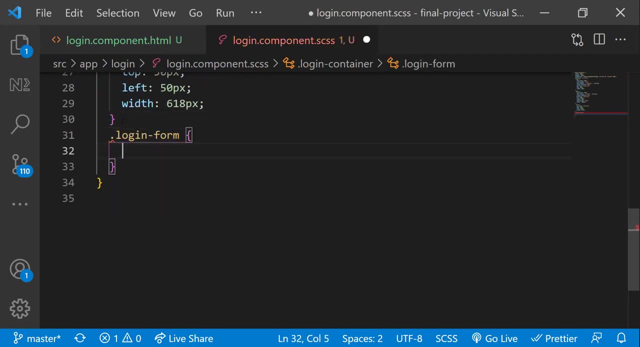 In the first two form group, let me add a label and an input text. Let me also create the password field in the next two form group. Okay, I'm going to position the form and apply some styles For the login form. let me give a width of 500 pixel and height of 300 pixel. 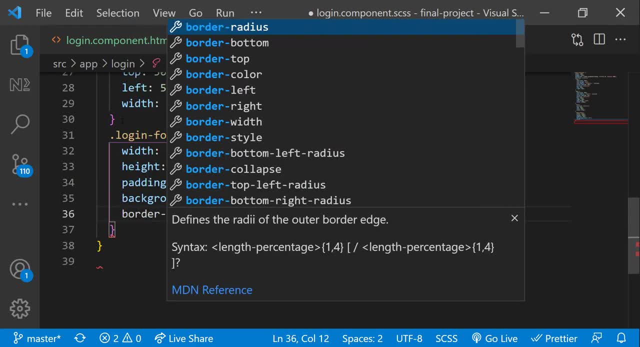 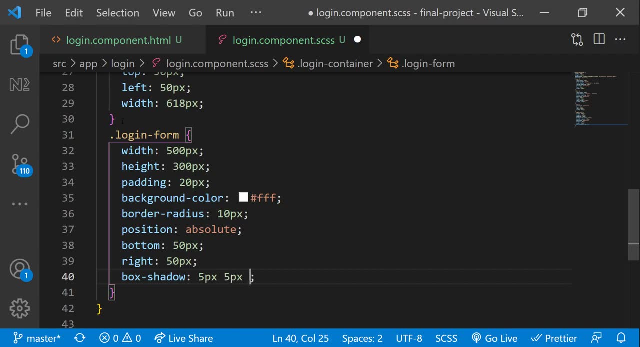 A padding of 20 pixel. background: color: white border radius: 10 pixel. position: absolute width: bottom: 50 pixel and right 50 pixel. I'm also adding a box header. Okay, Form control class is missing in the controls. 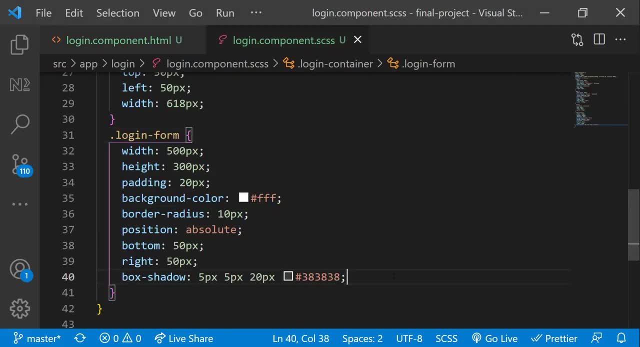 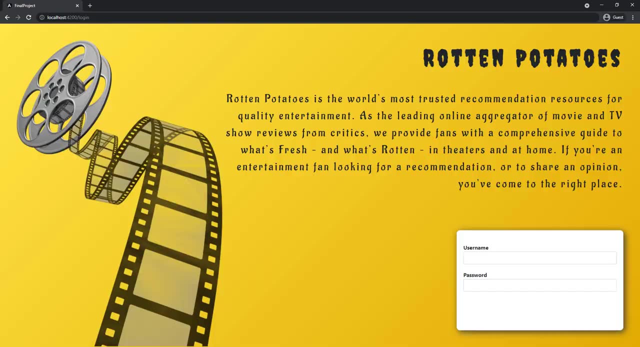 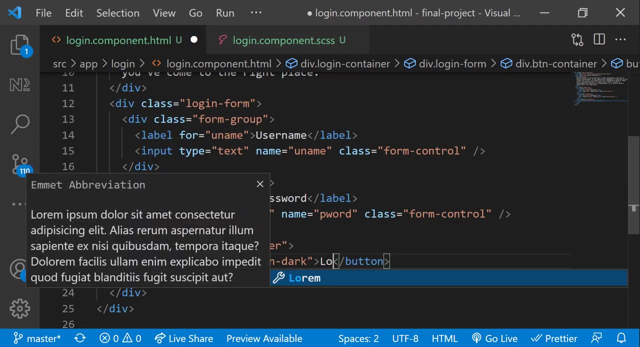 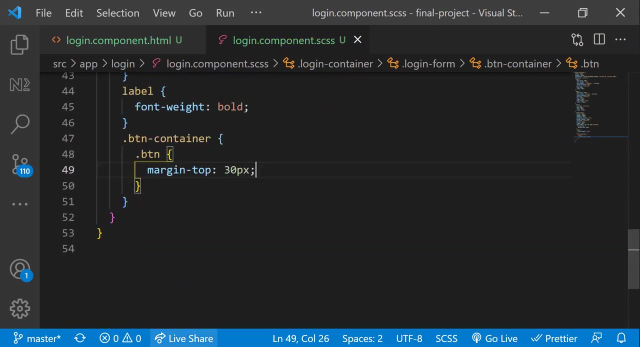 Now looks good. Let me also add a margin to form group and highlight the labels. Now let me add the button and a margin to the button. Okay, The login page design is completed. Let me get into the functionality. Ideally, I need to get the user name and password. 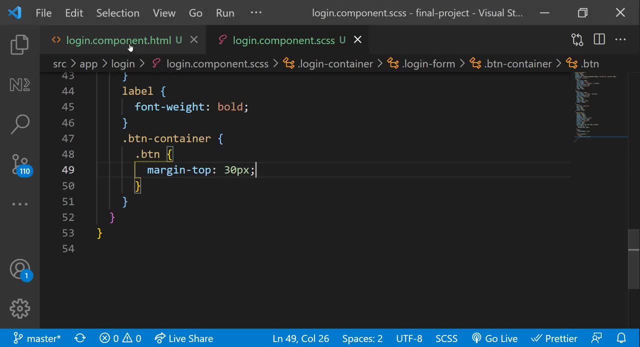 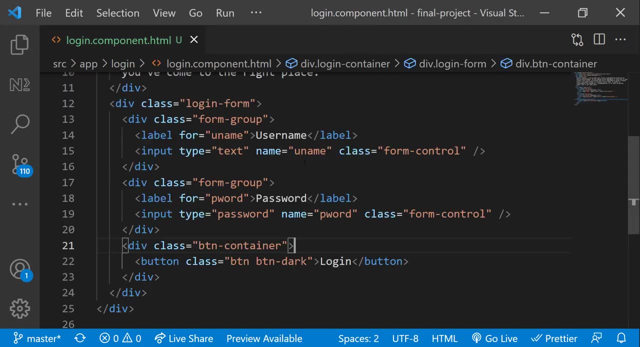 And validate against the database. but I have not set up any database, So let me make it simple For now. I can hard code the username and password inside the code. To get the username and password I can use the data binding concept we learned. 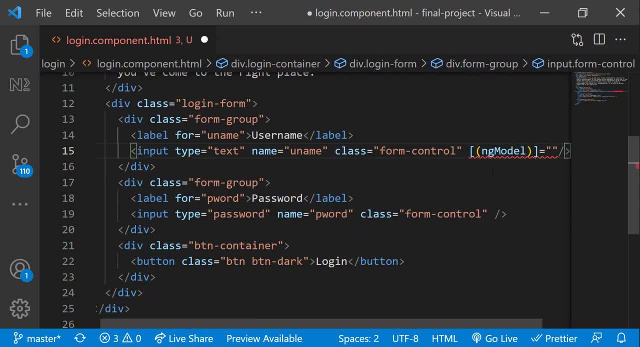 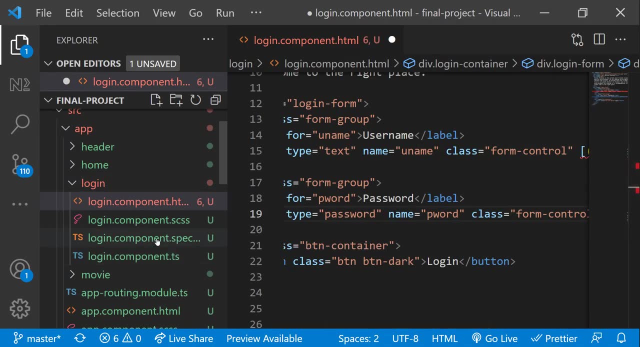 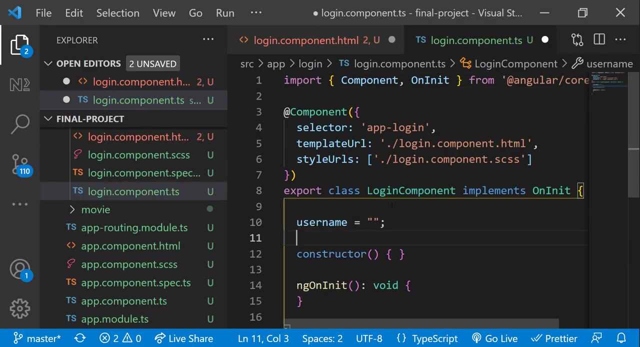 Let me use ng model Two way binding. To use ng model: first I need to import the forms module in the app module. This is an easy way to use it. I will suggest that I use the何n module. You can use other modules to get the code. 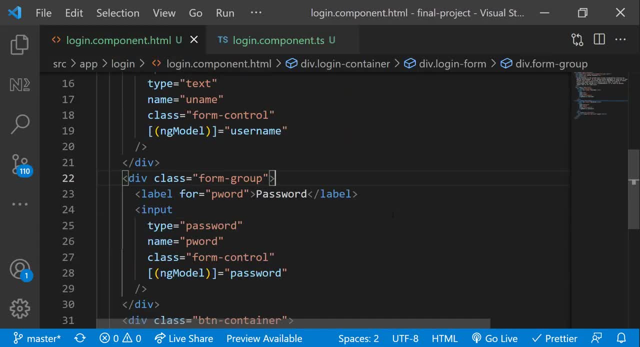 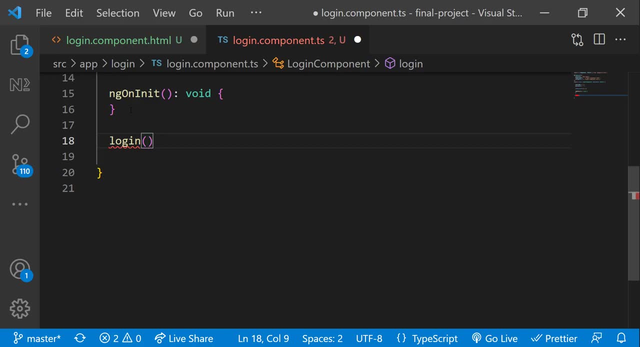 But it is best to use the ones I have in my company. Let me add a function called log in to log in And I will assign some function on the login function. For example, I will also add a function in the login function. 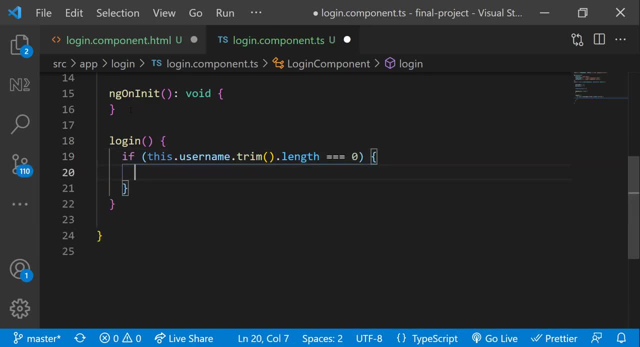 And what does that let us know is that I am going to set up a function that will allow you to add a message to the login. Now, I won't be doing any more КМ. I will be adding a function And here. Well, let's go ahead and make this. 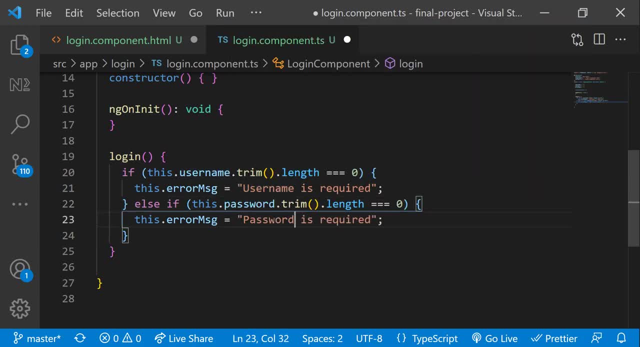 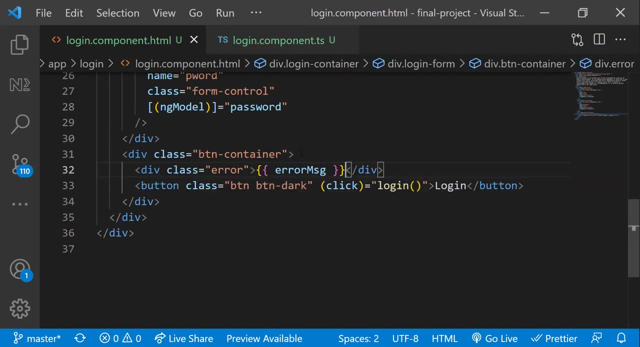 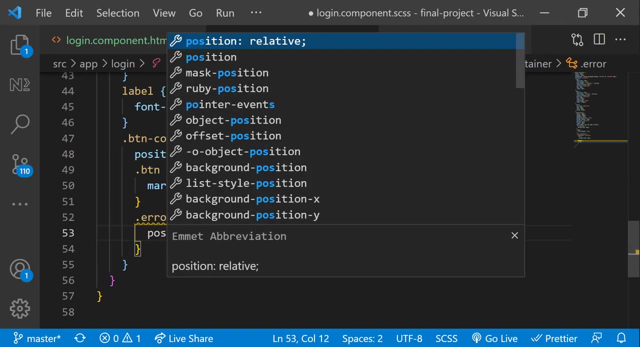 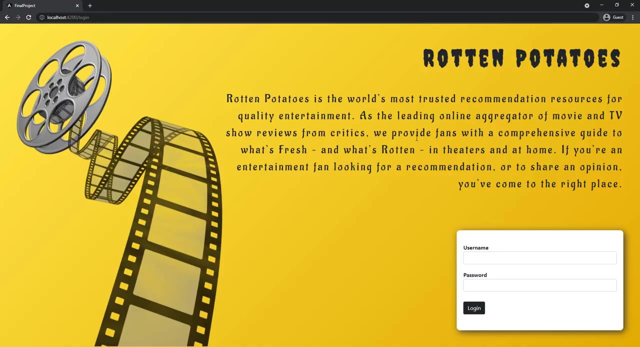 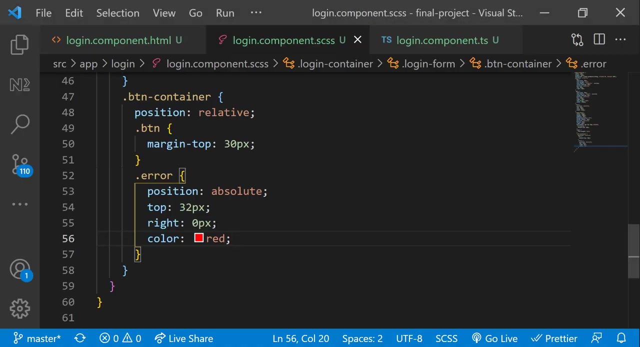 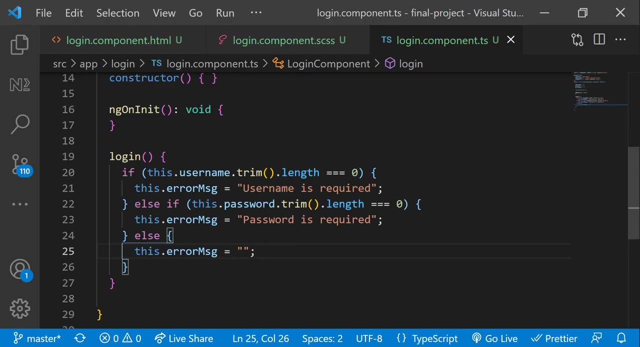 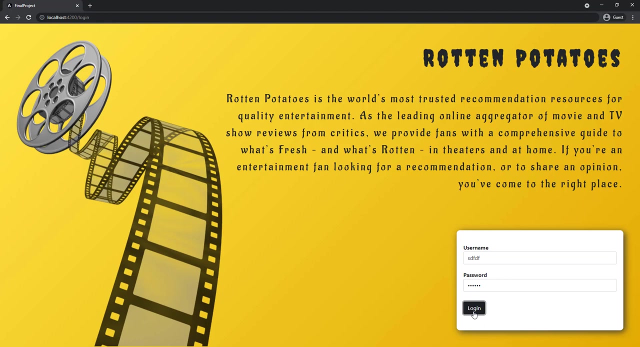 And display that in the UI somewhere here. So in button container I can use string interpolation to show the error message. Let me also add some styles to position that. Okay, let me test that once. Fine. now when the validation is passed, I need to route the user to home page. 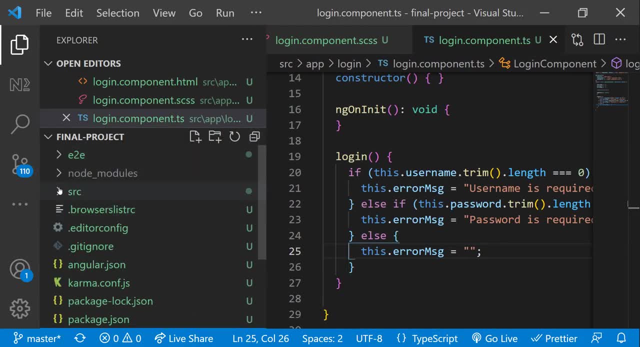 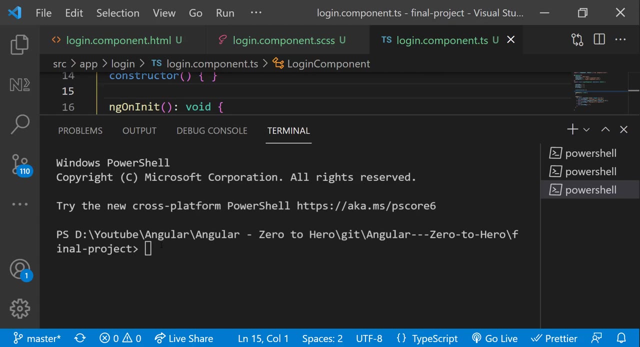 But here I can make use of service to group all the authentication related functions and keep it in a single place. Let me create a folder. Let me create a folder to group all services Inside the folder. let me create a service using CLI NGGS service name. 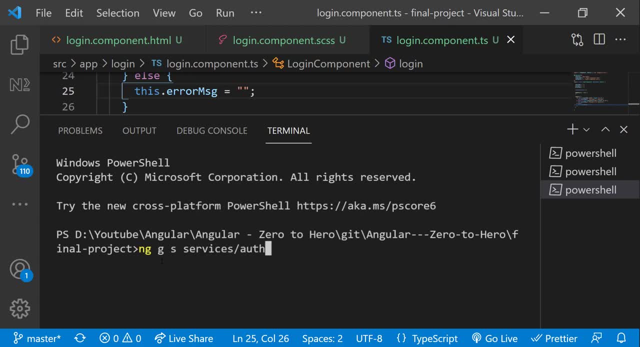 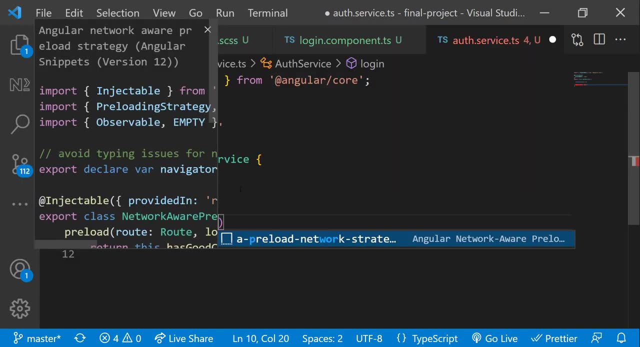 Let me give it as auth And I need to specify the folder so that the service will create. inside the services folder In the authgut service, let me create a function, login- which accepts both username and password. Let me hard code the logic here. 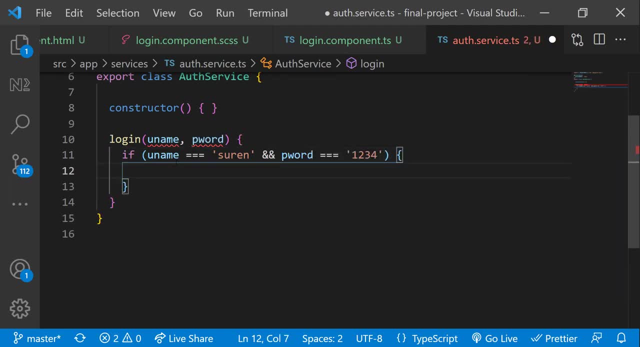 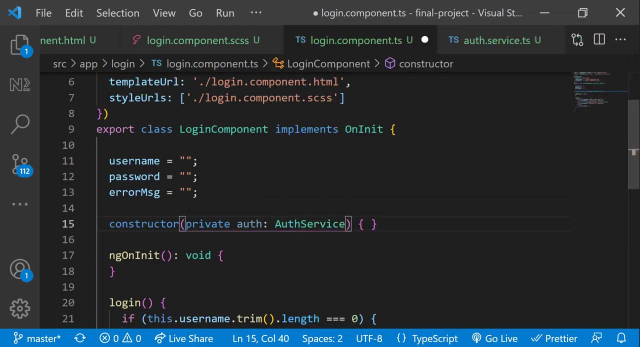 If the username is my name and password is 1234, return a success- code 200.. If not, let me return an error- code 403.. And in the login component, let me invoke the function in the auth service For that. let me inject the auth service in the constructor of the login component. 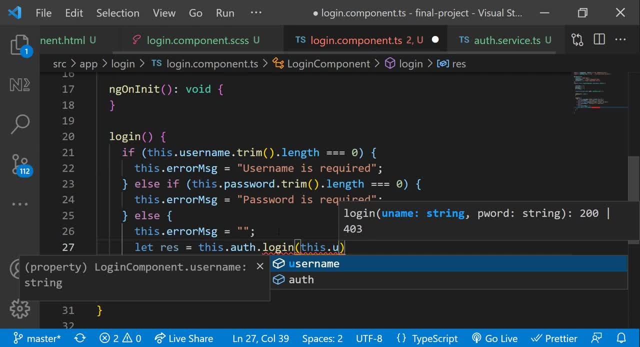 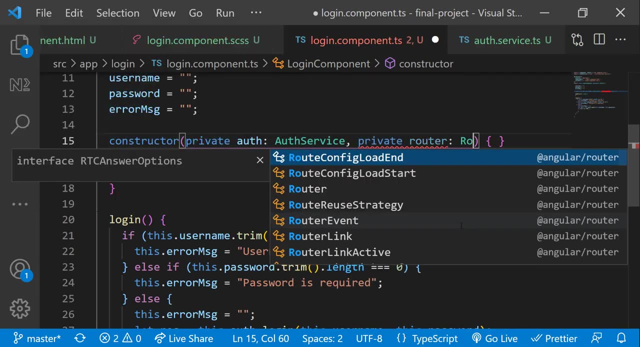 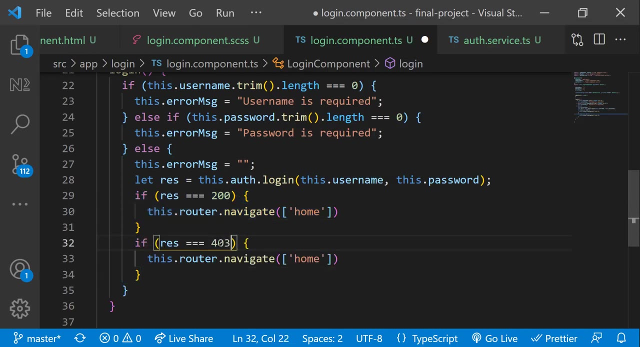 And then I can use it like this: I can route the user to home page using the navigate function in the router. Let me inject the router in the constructor And then I can use it like this. And now, if the response is 403, I can show an error message. 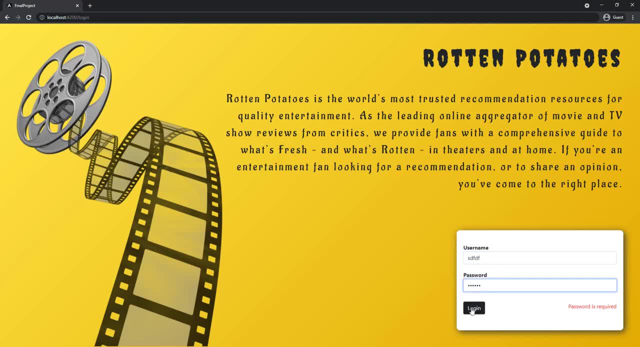 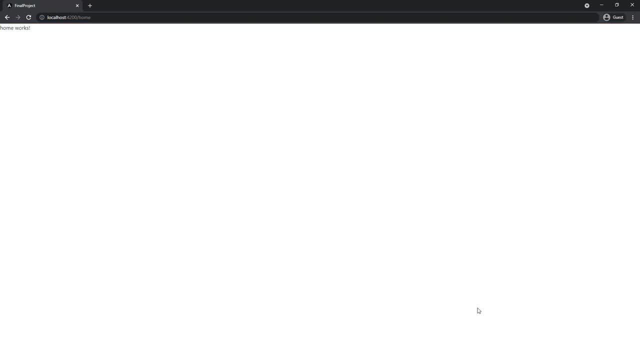 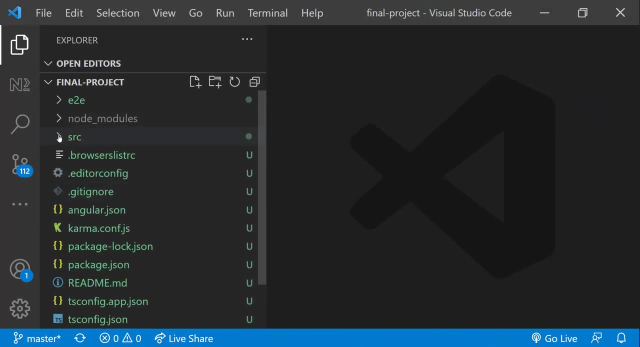 Let me test this once. Okay, It is working. I am going to move to the homepage design. In the homepage and in the movie page I have a header which has a link And I edit it in my nous� Page And then I go to the home page. 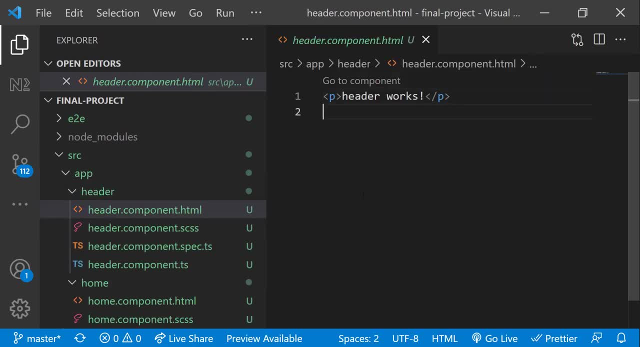 I edit it in my nousæ Page And then I shown the task 라고 the image on which all the homespaces has appeared. Then I go to the page And then I show the task be a common component. so let me start with the header design in header component html. 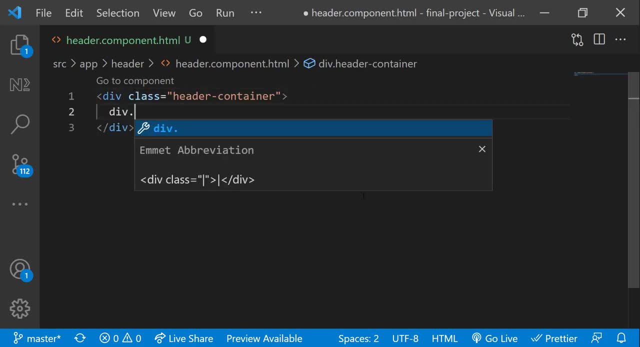 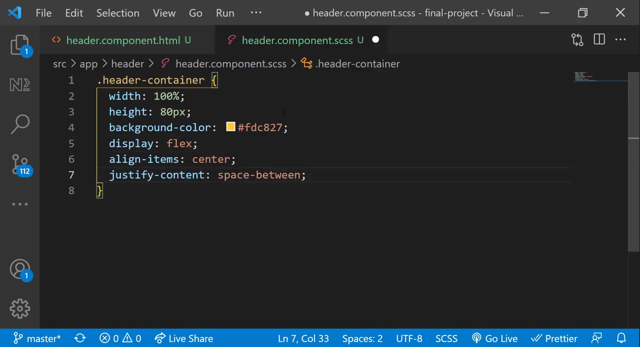 let me add a header container and inside that a view for logo and another div for logout. in header component css, let me add a width of 100 percent height, 80 pixel. background color of dark yellow display flux, align item center and justify content space between now, let me. 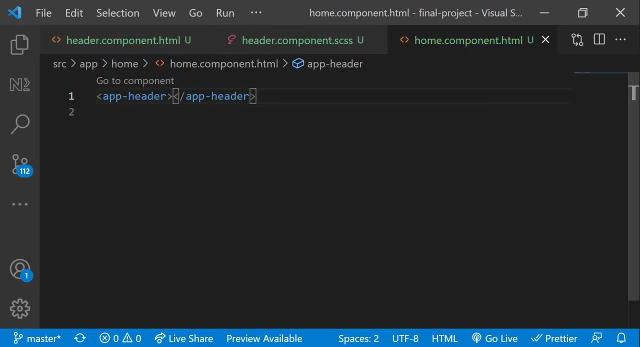 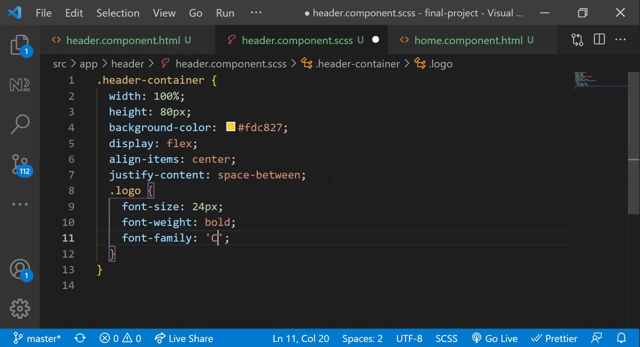 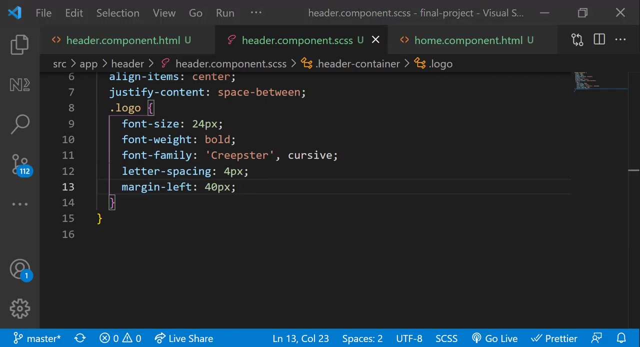 add the app header in home component and so i can preview that. okay, now for the logo, let me add font size: 24 pixel. font width: bold font family creepster letter spacing: 4 pixel and margin left: 40 pixel. okay, and for the logo, let me add font size: 18 pixel: foreign black bold. 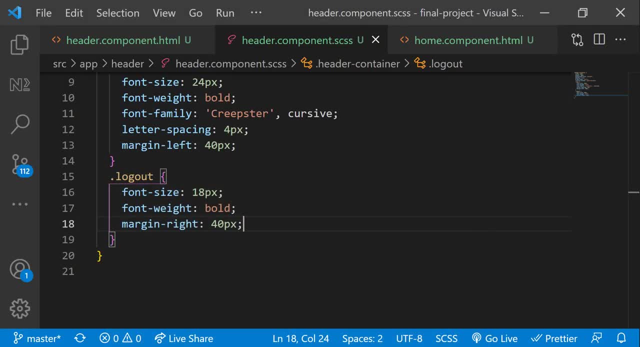 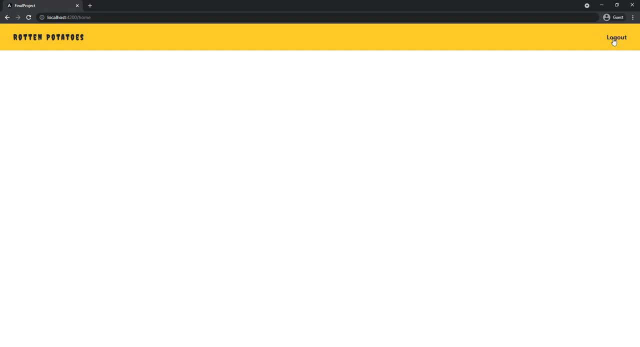 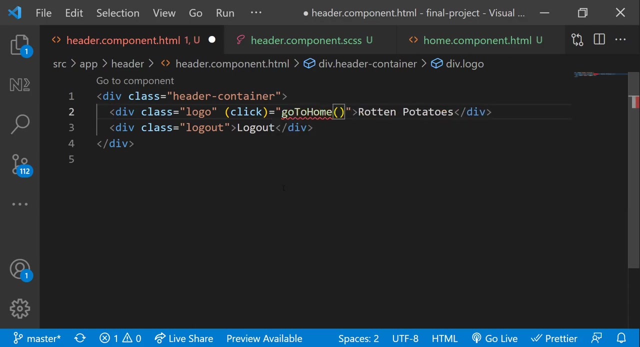 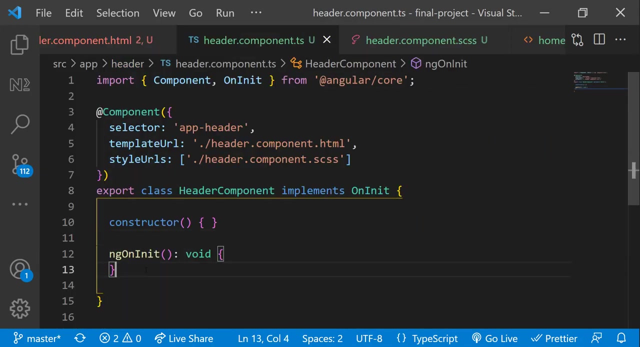 and margin right 4. Okay, looks good And I'm going to add click events to these two. So let me add cursor pointer to both so that it appears clickable, And in the header HTML let me add click events and create those functions. 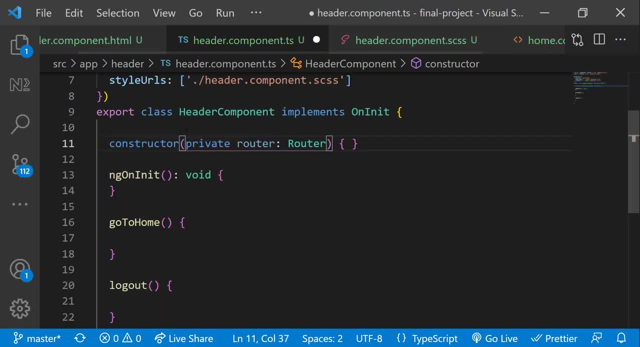 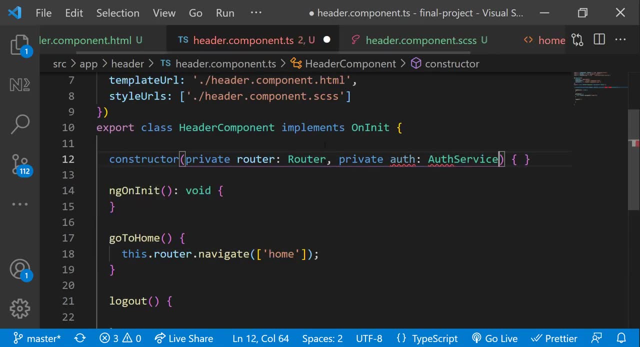 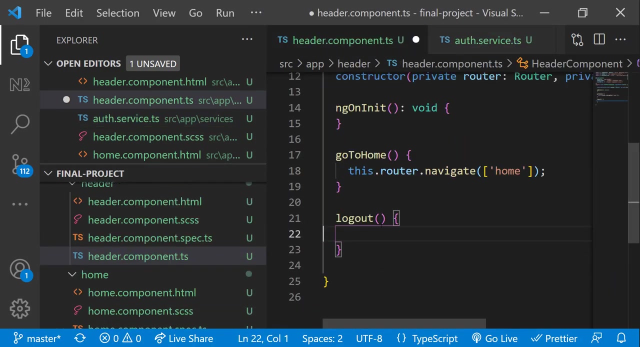 For go to home, I can use router to navigate to home page. so that I can easily navigate to the home page by clicking the logo. And for the logout, let me inject the auth service and call logout from there. Let me also create that function in the auth service. 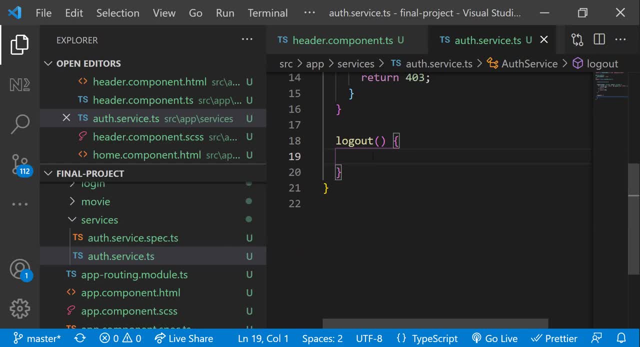 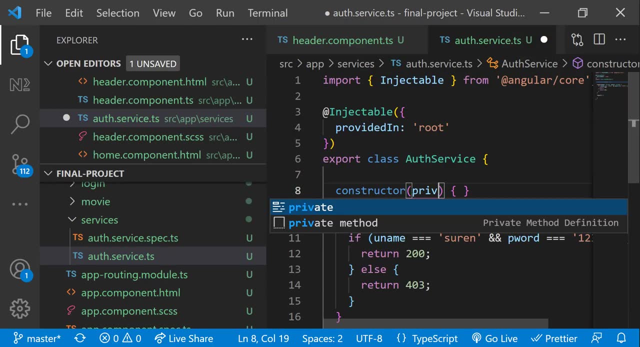 Usually when we integrate with the real authentication system, we sometimes call the logout API of that system to invalidate the token. Or sometimes we clear the token And then we call the logout API of that system to invalidate the token, Or sometimes we call the locally stored authentication information, like token etc. 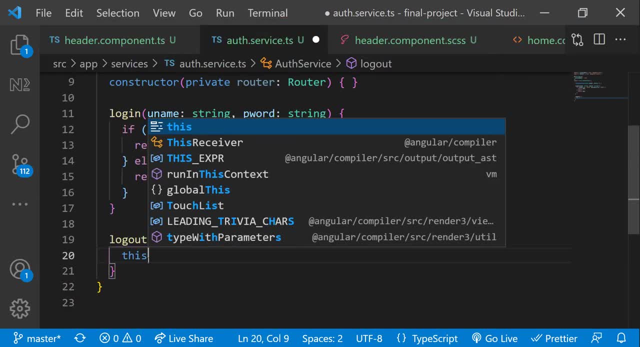 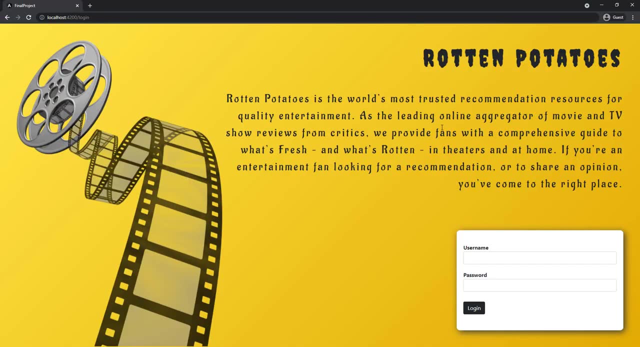 And then route the user to the login page. But here, as I have already mocked up the authentication process, I can simply route the user to login page. Okay, let me test this. It is working as expected. Let me continue with the home page design. 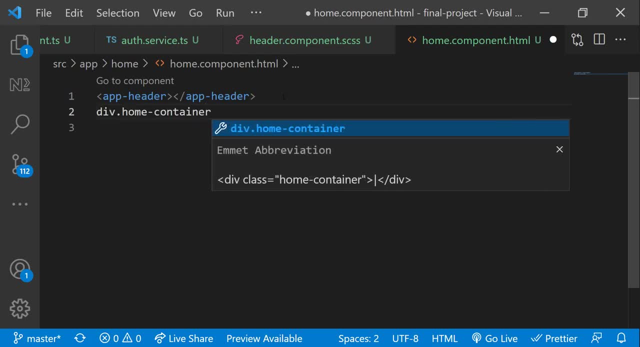 In the home page HTML after the header. let me create a home container Inside that. I want one section in the left and one in the right, So let me create two divs: 1. all movies and other one for showing popular movies. 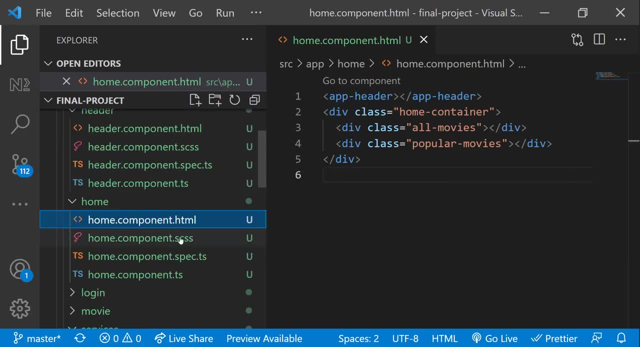 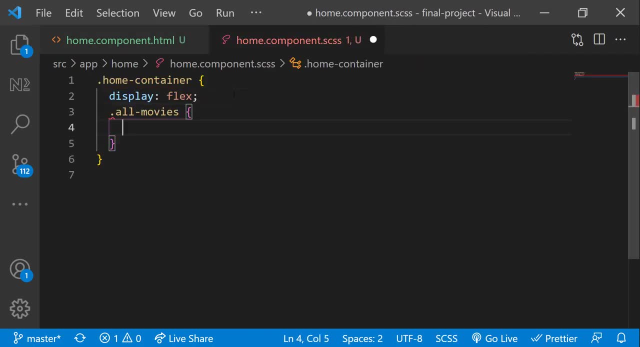 In the CSS. let me add some styles For home container. I can add display flux so that the divs inside that come side by side. For all movies, let me add 75%, and for popular movies, let me add 25%. And for both the divs, let me add a min height calc of 100bh minus 80px, which is the height. 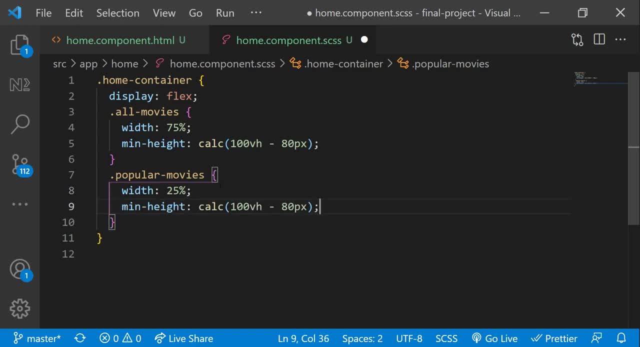 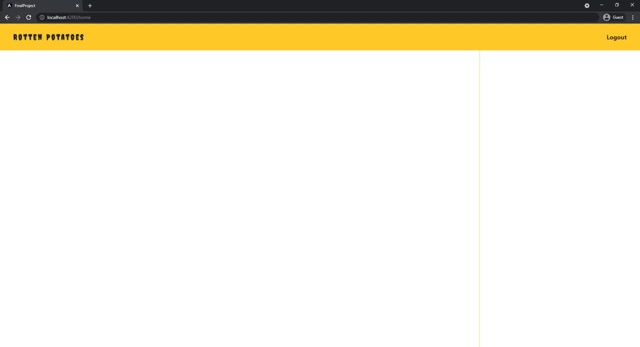 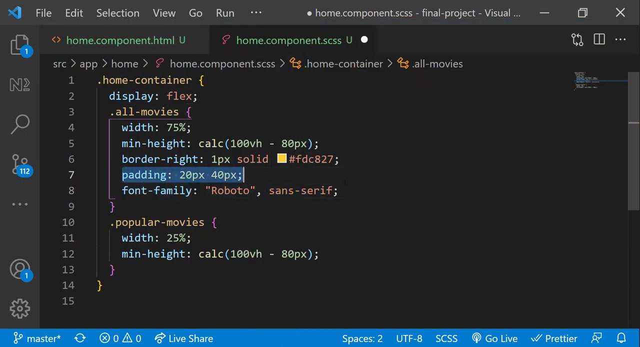 of the header so that it occupies the entire height of the viewport, And then let me add a border right so that I can see a separation. Now let me add a padding and font family to both. First, I am going to start with trending movies section. 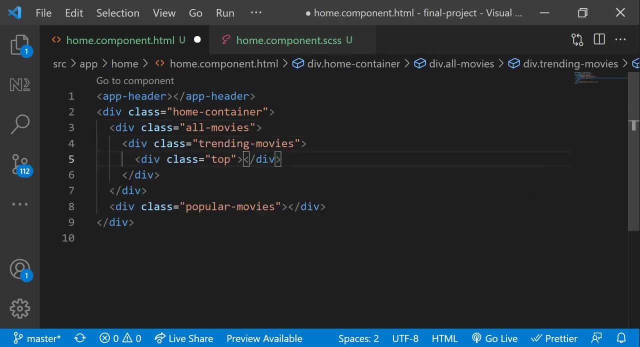 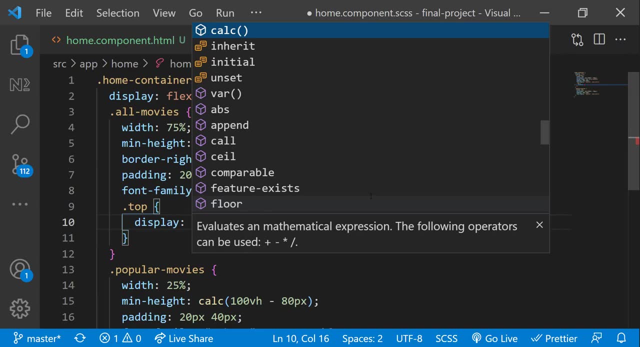 Let me create a div for that. Inside that I need a top section where I can display a header- trending movies- And view all button. Let me style this first. So for the top, let me use display flux, align item center and justify content. space between. 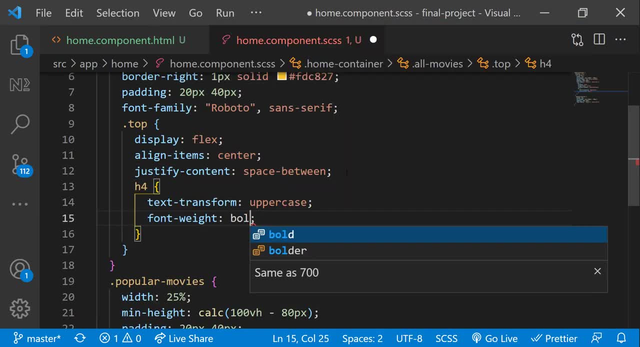 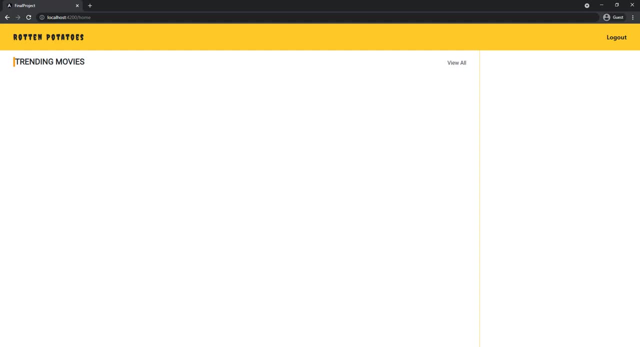 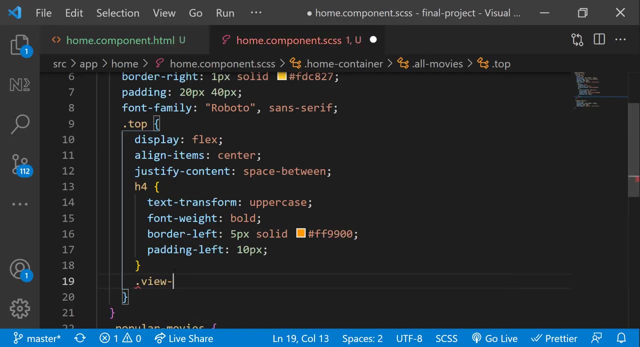 For the heading tag, let me add text transform: uppercase font weight bold and border left: 5px solid yellow. Let me also add a padding left. Ok, now for the view all, let me add the same color and cursor pointer. Next, I am going to create a div. 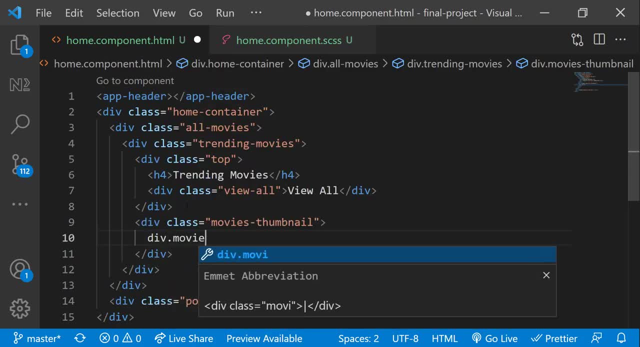 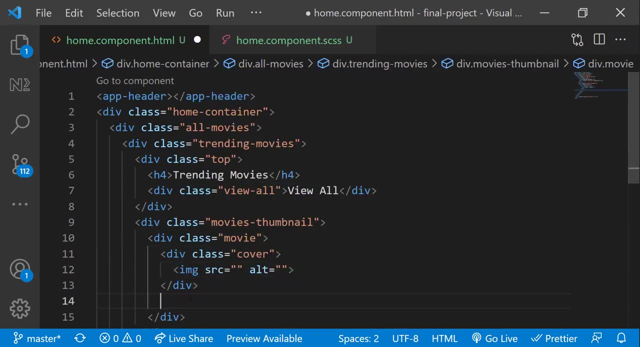 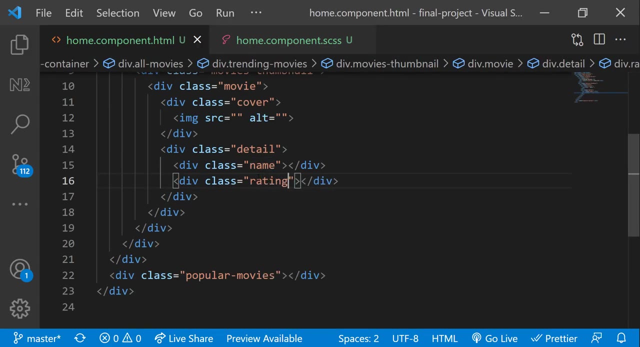 To display all the movie thumbnails Inside that. I am going to create divs for each movie. Inside movie div, I need a div for movie cover image and then another div to hold movie details, name and rating. Before applying styles to this, let me explain how we can get data for this. 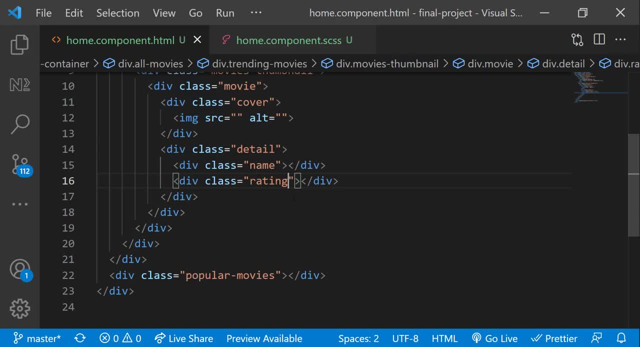 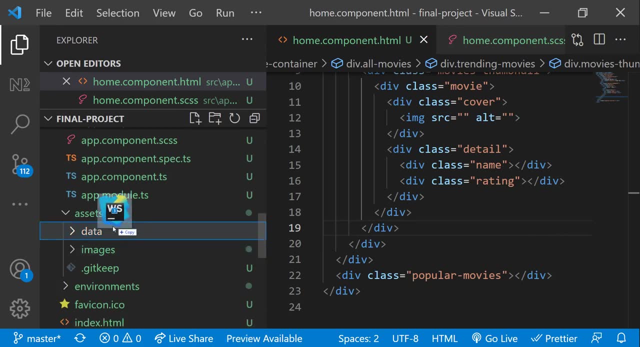 As I have not set up any database, I can mock up the data I need using json in the assets folder. For that, let me create a data folder inside assets folder and copy the json I have created. Usually we get this kind of response from api. 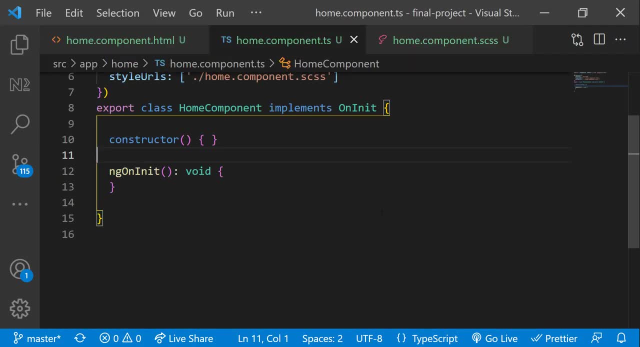 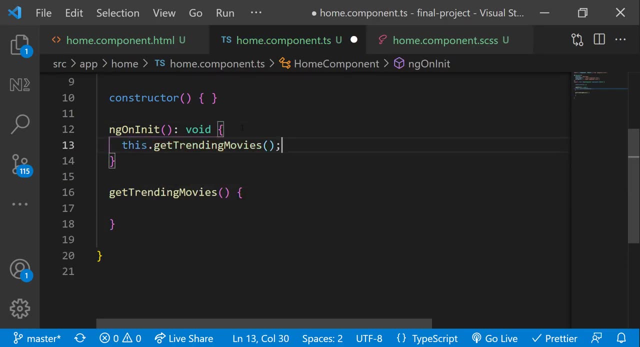 But now I am going to get this json using http. So in the ts file let me create a function And I am calling this function in the ngOnInitHook. Inside that function I am going to use http client to get the json For that. I am going to inject the http client in the constructor. 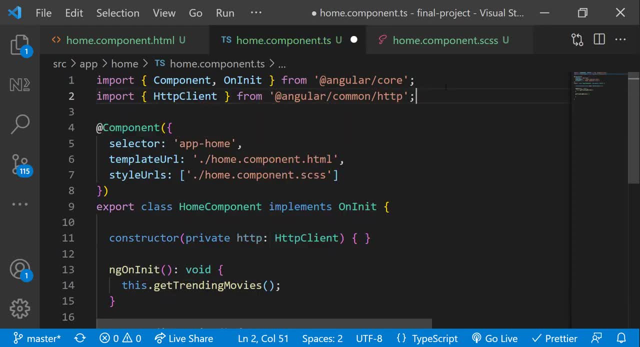 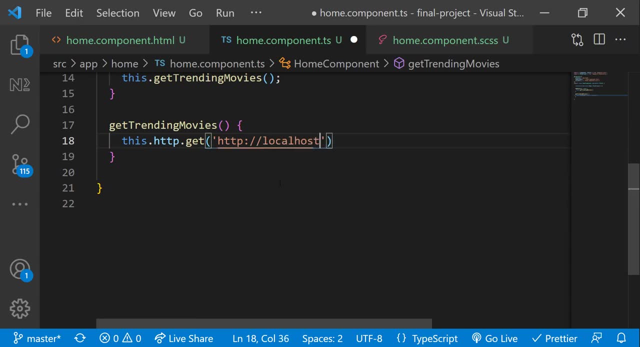 I can import this http client from at angular slash, common slash http. So now I can call the get method of http. Which exception is there? Ok, Let me give the url, Let me give the localhost url, And I believe you remember that we need to subscribe. 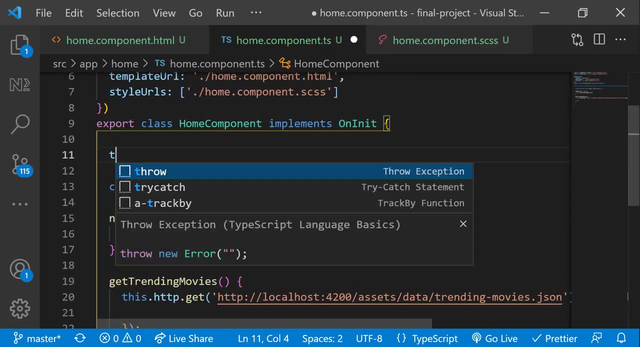 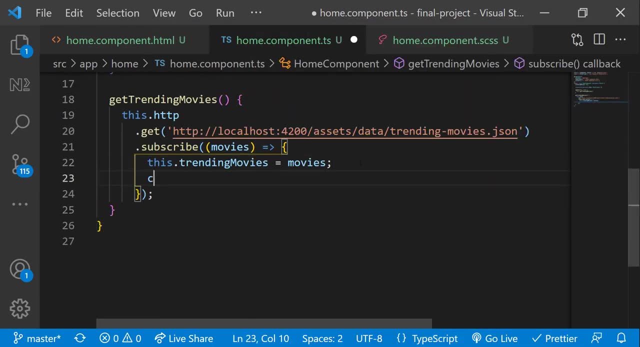 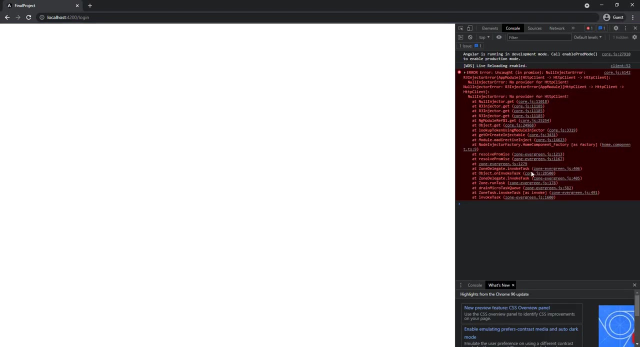 Only then we are able to get the data. Let me create a variable to hold the trending movies and assign the response to that. Let me console it so that we can see the response. I think everything is completed, Is it? No, I missed one thing. 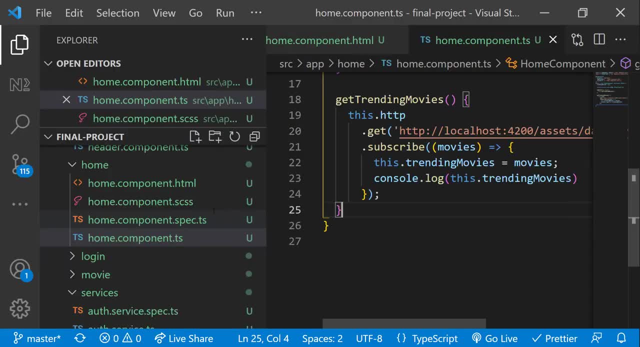 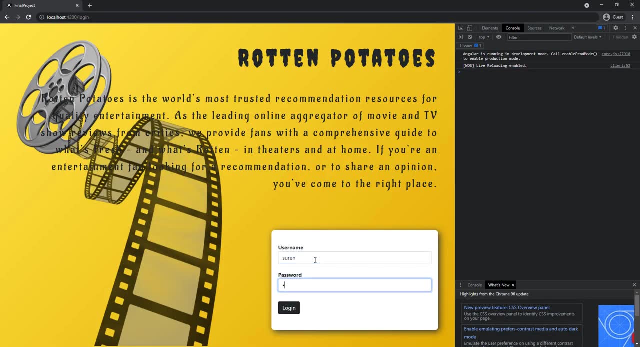 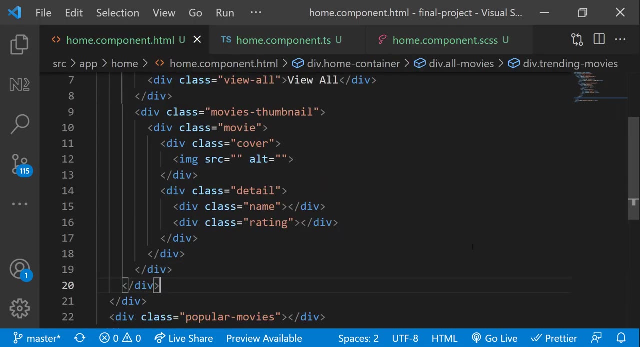 R3 injector error. Do you remember what I have missed? To use the http client, we need to import the http client. Let me import that. Now we can see the response. I am going to bind this first with the html. First let me use ng far. 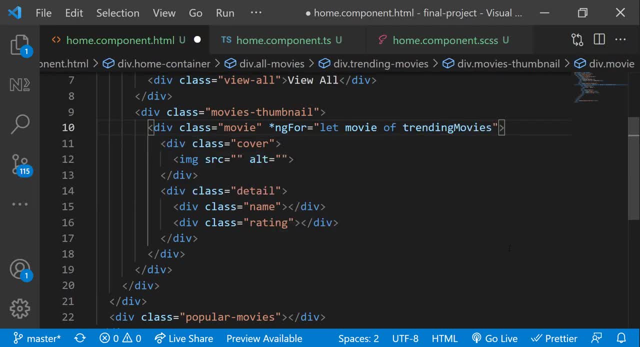 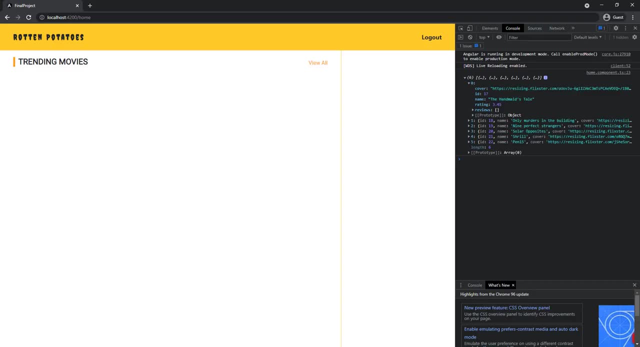 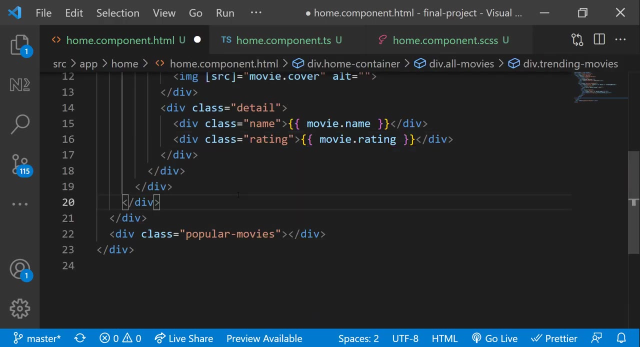 Let movie of trending movies Inside the cover div. I am going to use an image tag in which I am going to use property binding to bind the source And I am going to replace the name and rating with the right values. Now we could see this. 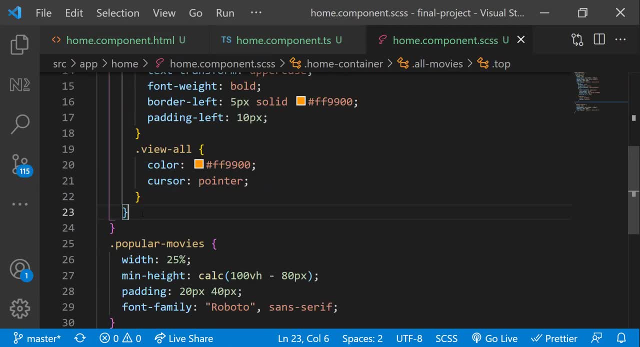 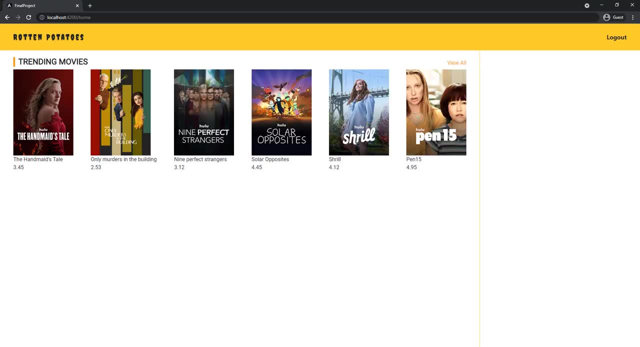 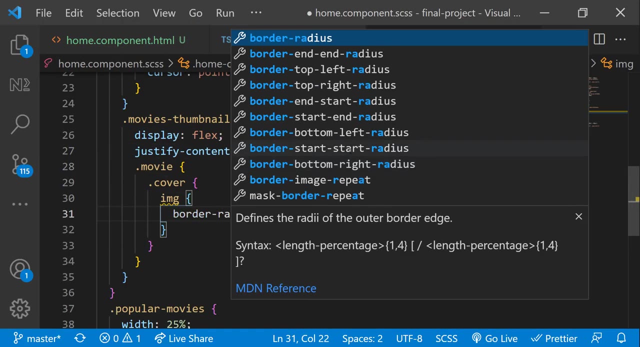 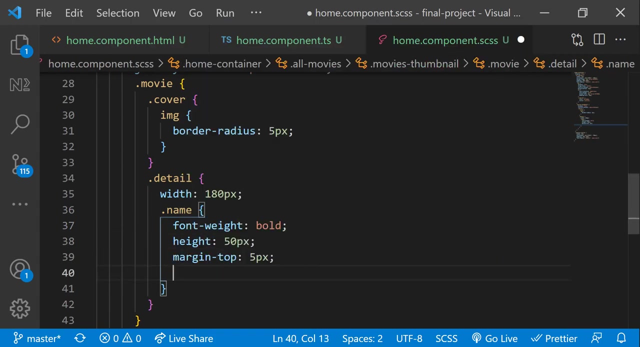 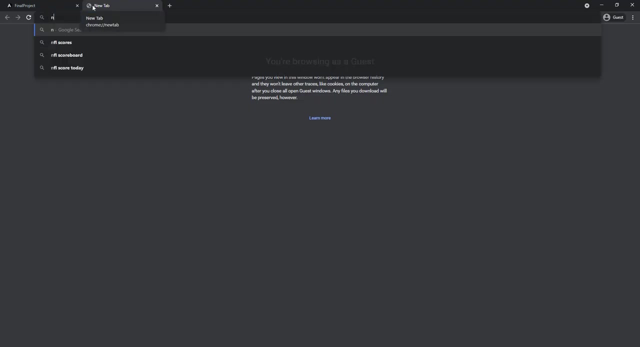 Let me apply some styles For the movie's thumbnail. let me add display flex and justify content space between. Let me give a margin bottom to top section And I can also apply some styles to the movie div. Ok, Looks good For rating. I am going to use an angular library ng bootstrap. 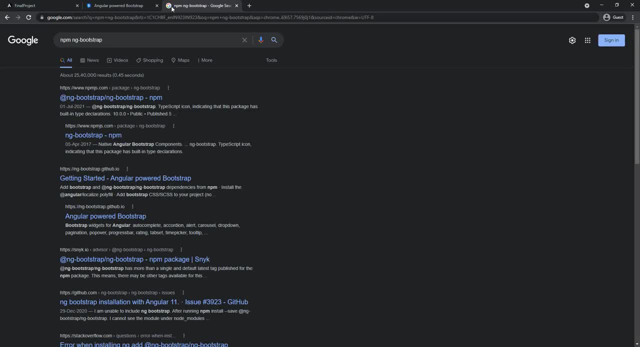 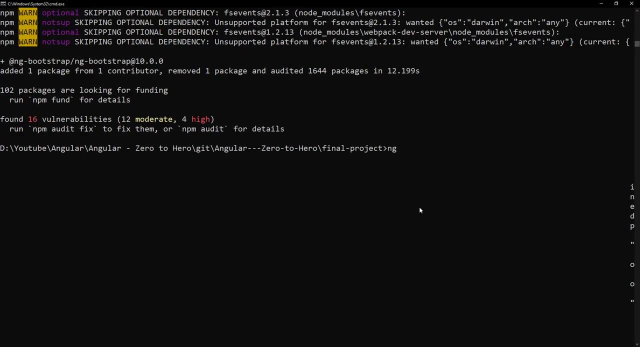 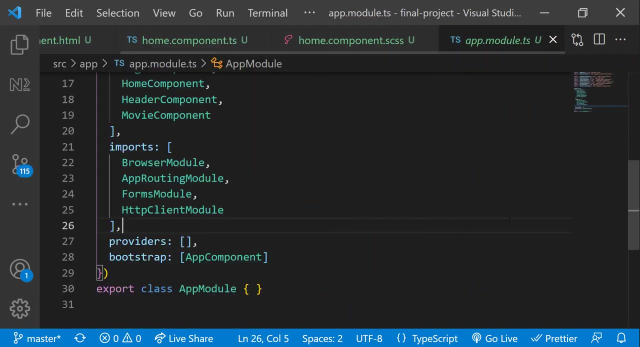 So let me install that. Let me stop the server for a while and install this. It is installed. Let me start the server again. Now I need to import the respective module To know about how to use that library. we can refer the documentation of that library. 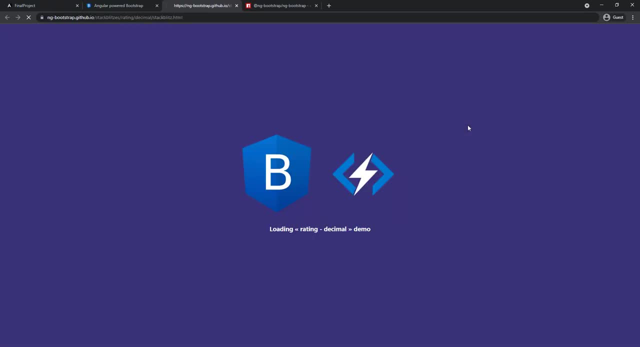 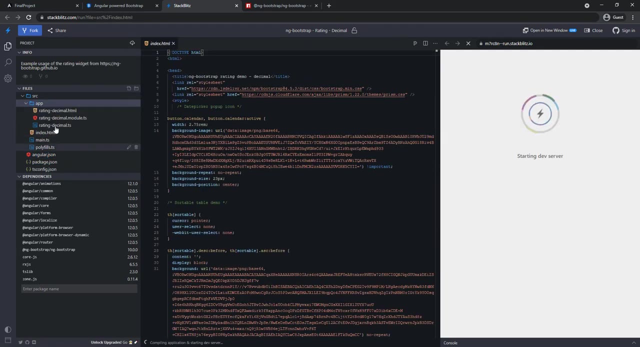 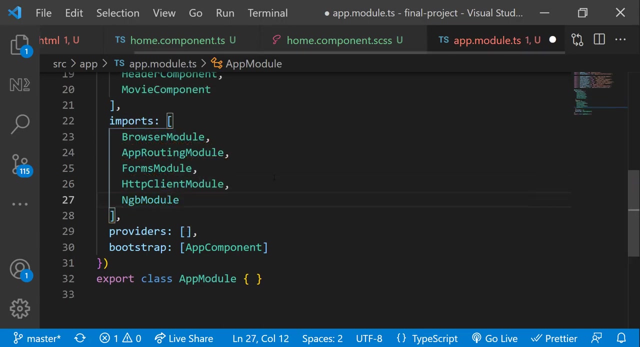 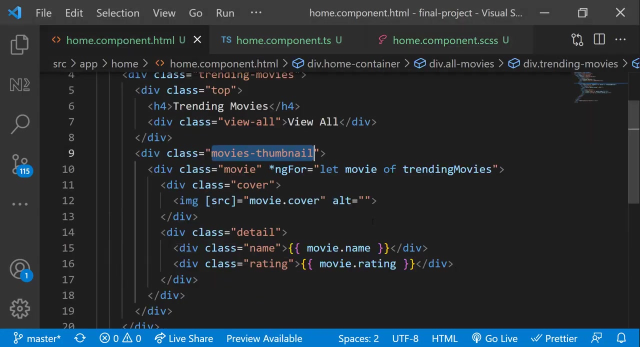 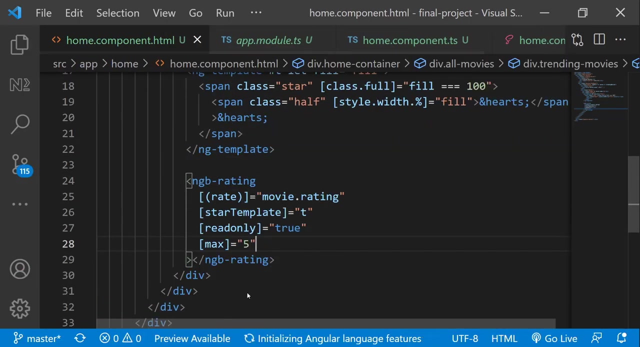 I left it as it is. Ok, I like to use this one. Let me open the stack blades- Ok, We can use this. And let me pass the right rating field- Ok, It is showing like this: I think I haven't added the CSS. 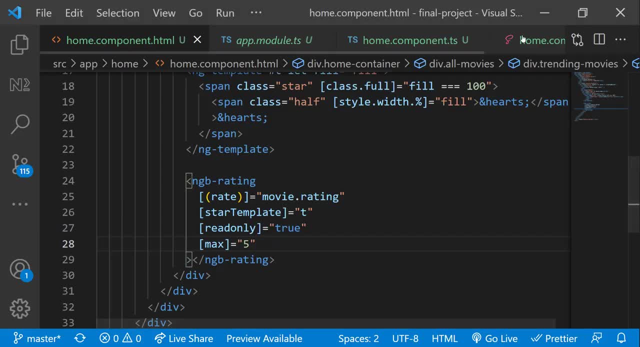 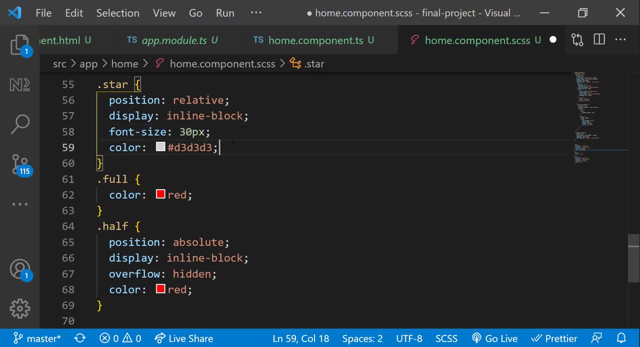 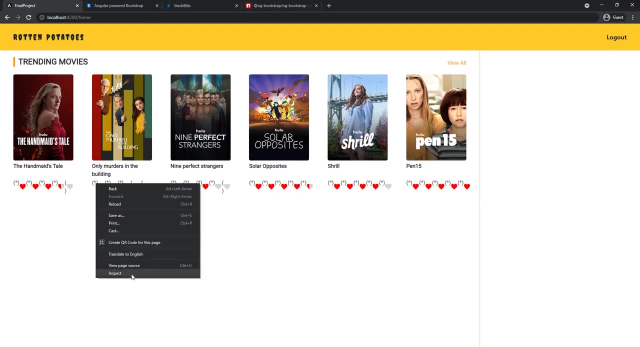 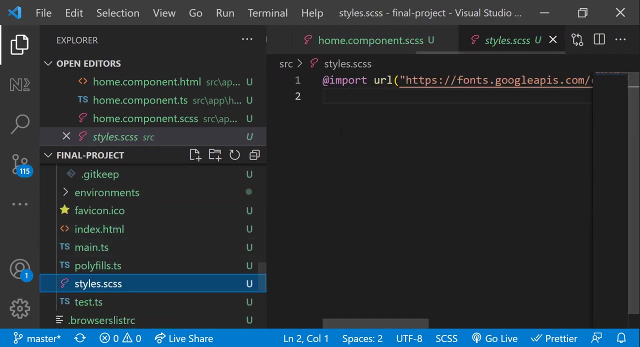 Let me check. Now it is showing like this: Let me change the font size and add a different font. I guess this library is not optimized yet for this angular version. I don't need this extra text. Let me hide this. And when you modify some library styles, you need to put the CSS in the global style CSS. 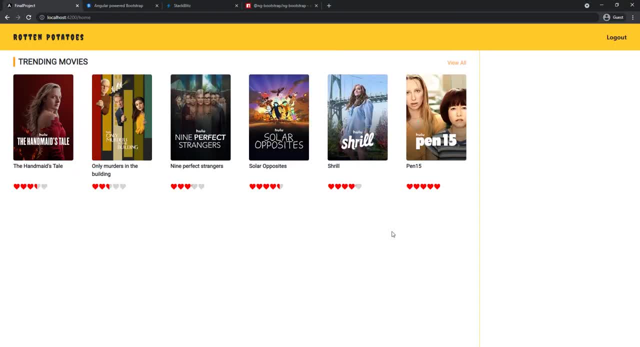 Only then it will reflect. Ok, Now it seems to be good. Let me give a margin right and a height. But it should be good if we create this rating component as a separate component, So that we don't want to have all these code everywhere. 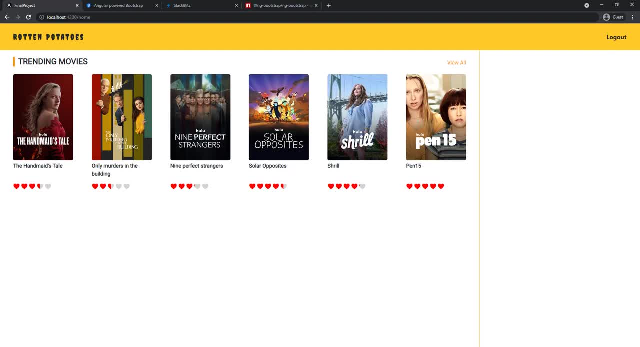 Also I am going to explain about modules concept in angular. Modules in angular are used for maintaining the modularity of the application. Modules are containers for grouping components, Services, etc. Based on our requirement. There are also lazy loaded modules through which we can reduce the build size and improve. 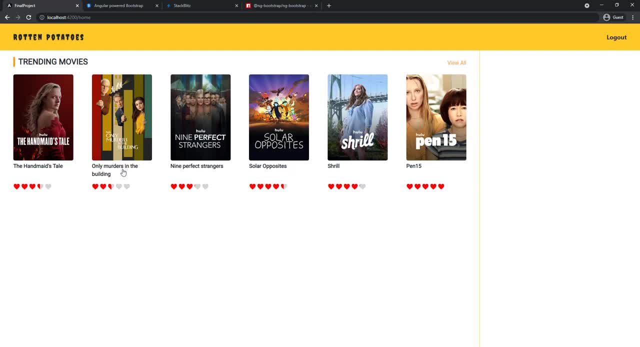 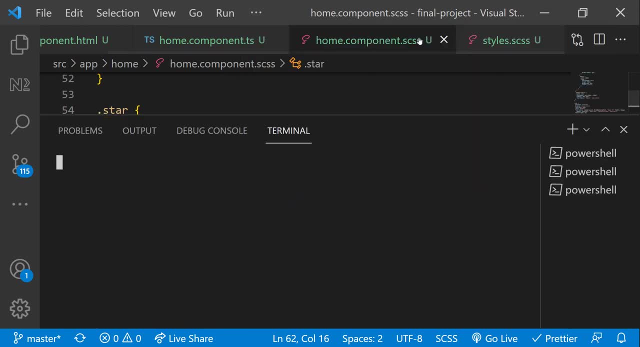 the performance of the application. I will explain more about modules, lazy loaded modules, etc. in the advanced course which is coming up soon. For now, I am going to create simple feature module where we can place all our components related to any feature. Let me create a module. 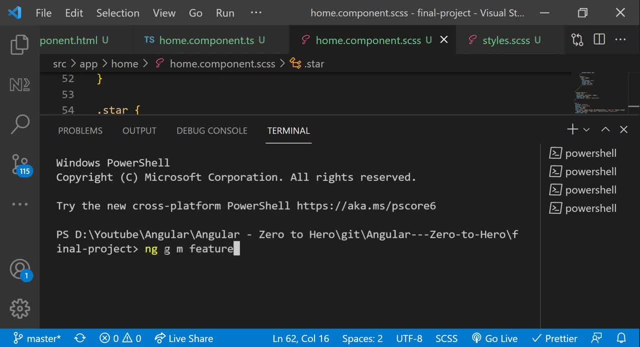 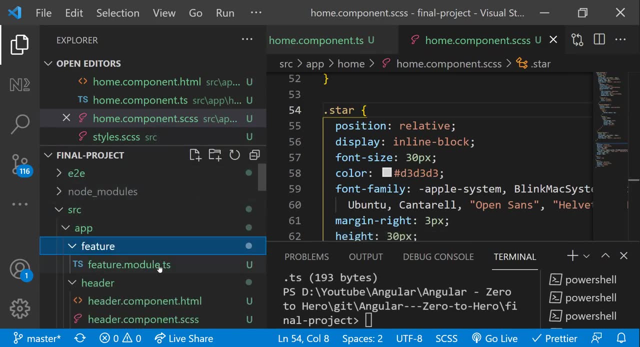 I can make use of the CLI ng-g-m module name. Let me name it as feature. Feature module is created And we can see it here Now, inside feature module. let me create a component for rating. Let me name it as star hyphen rating. 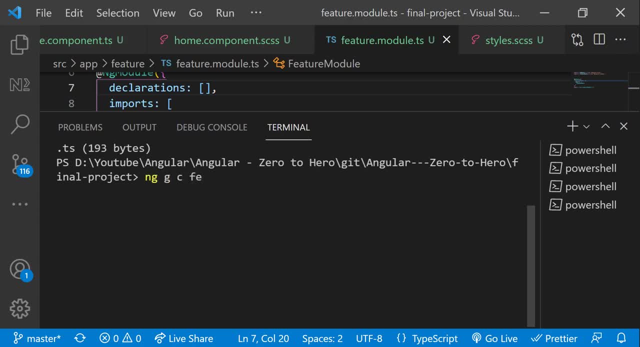 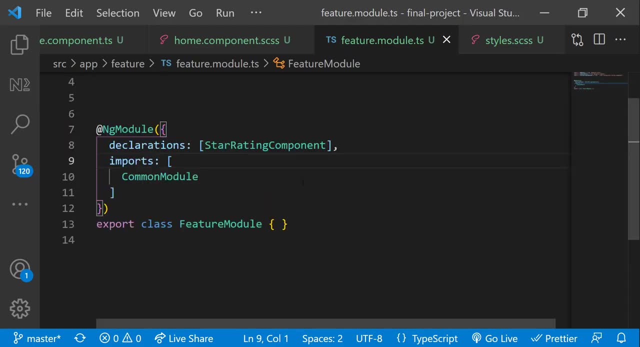 ng-g-c. this time I need to mention the module name. slash star hyphen rating Component has been created inside feature module And we can see it is already declared in the feature module. But to use it outside this module I need to export it. 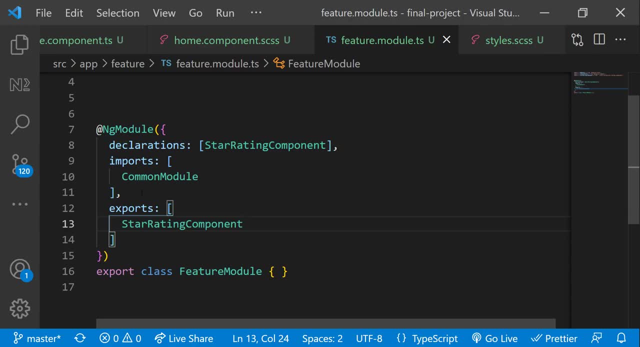 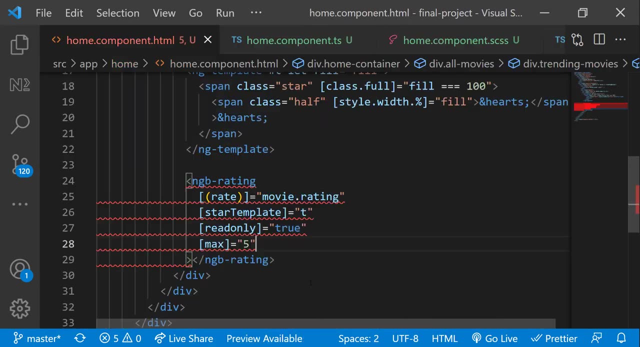 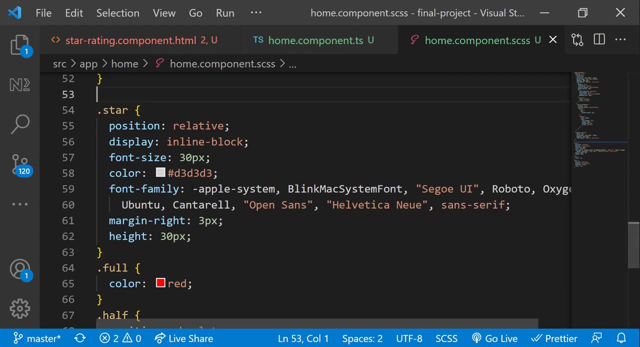 Let me do that Also. I have imported the ngb module in the root module. It is not needed. We can import it in feature module alone. Now, from the home component, I am going to take the rating related code and put it in the star rating component. 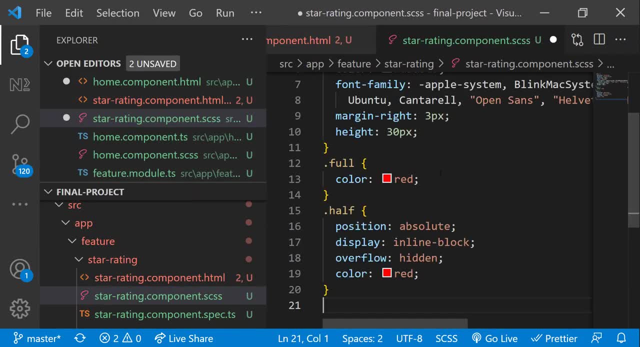 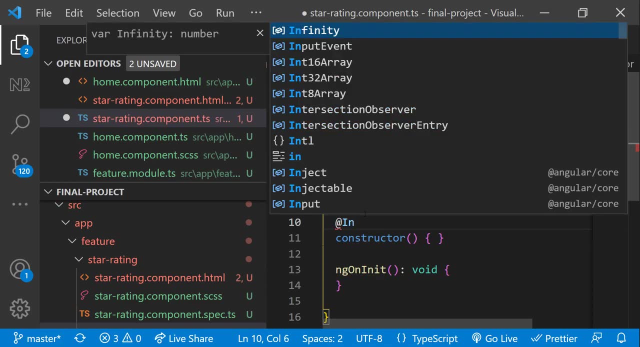 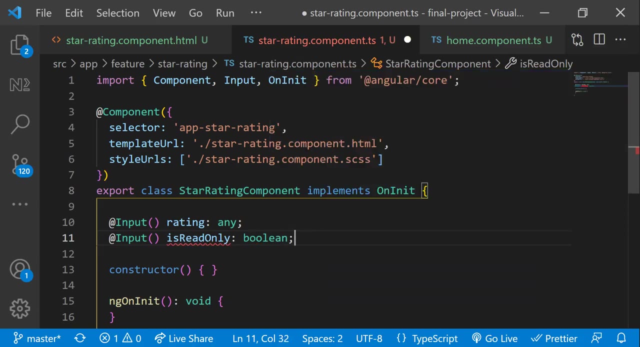 Also the CSS. Now I can get this rating value as an input to this component using at input decorator. Let me also get another property is read only, through which we can make this rating component Configurable. Now in home component, I am going to use this app star rating. 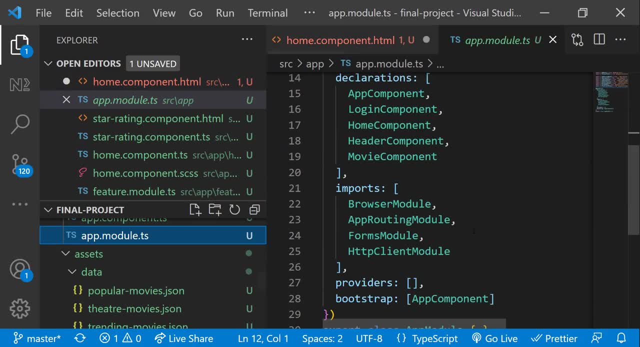 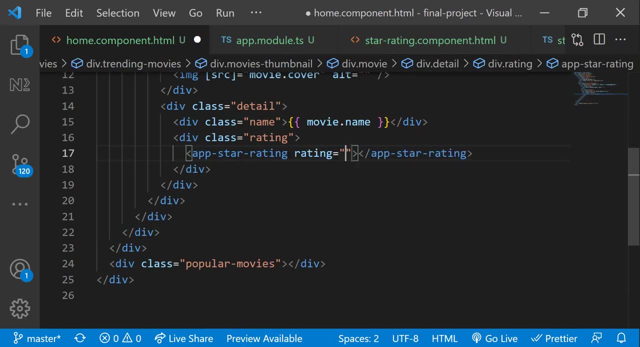 But it says it couldn't recognize this because this component is present in feature module. So I need to import this feature module inside app module so that I can use any component from feature module to other modules. Okay, now I can pass the inputs. It is working. 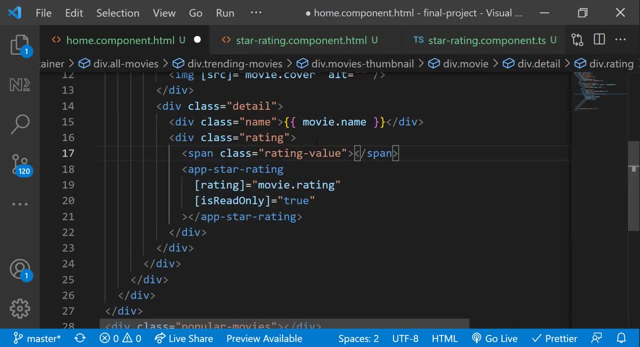 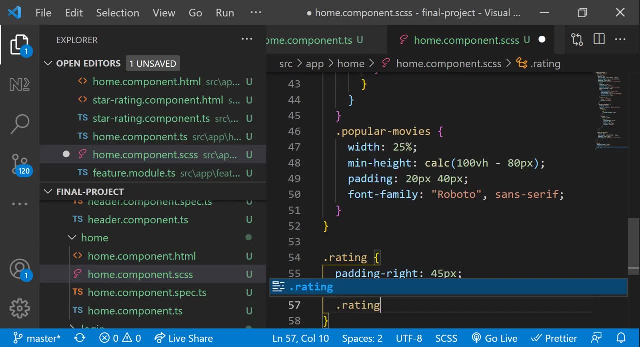 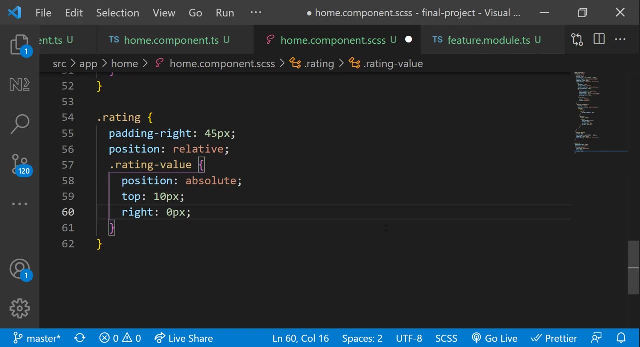 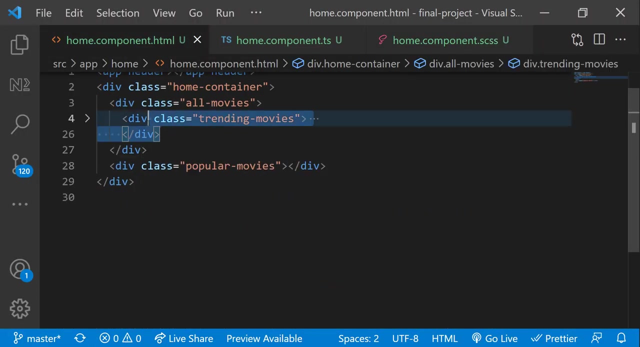 Let me also add the rating. Okay, Let me add the rating value For that. let me add a span inside rating div And then apply some styles to position that. Okay, looks good. Now I can copy the trending movies code and create the popular movies section. 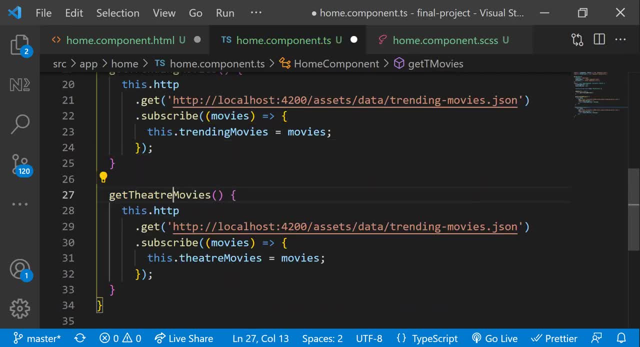 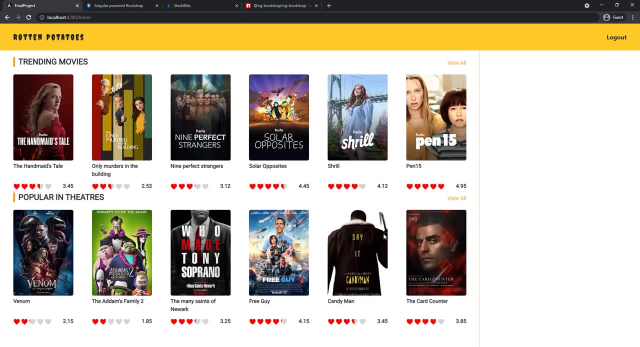 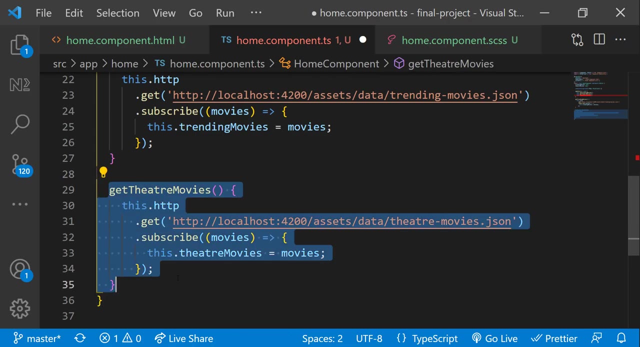 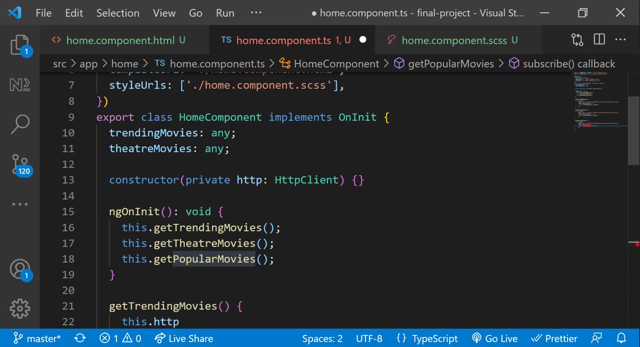 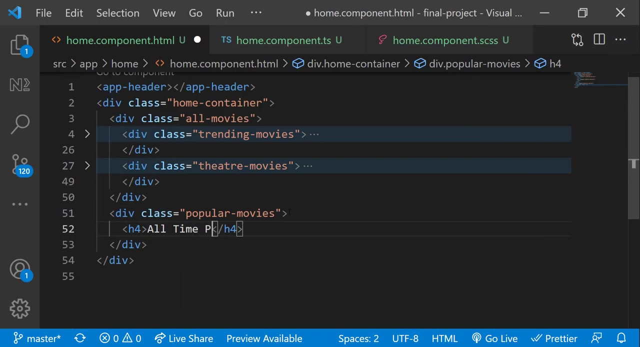 Let me add a margin bottom here. Fine, Let me also get the all-time popular movies list first, And in popular movies div, let me add a margin number. Okay, It is good. Okay, For the popular movies div, let me add a heading. 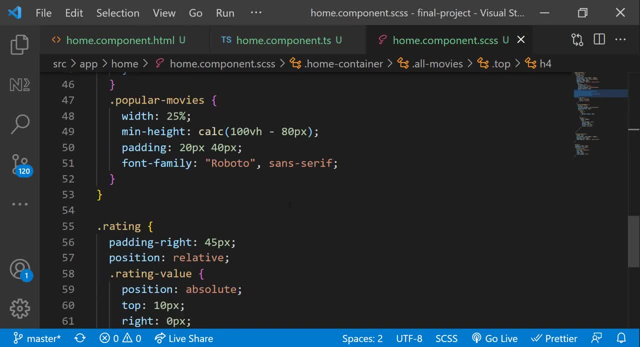 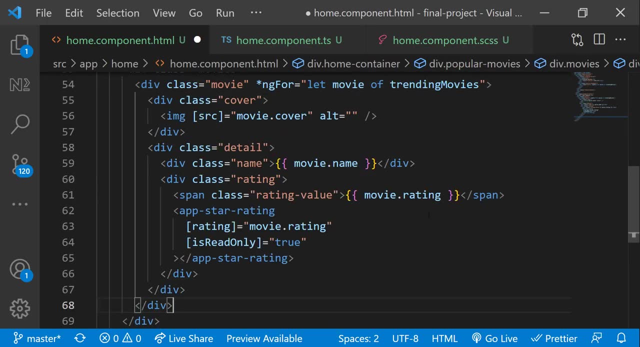 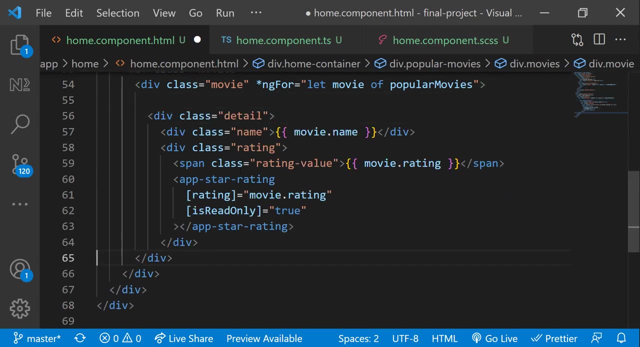 I can add the same styles as before And after the heading. let me add a movies div Inside that. let me copy the movie div from trending movies and change the variable name. I can delete the cover, which is not needed, and also the wrapper div, also not needed. 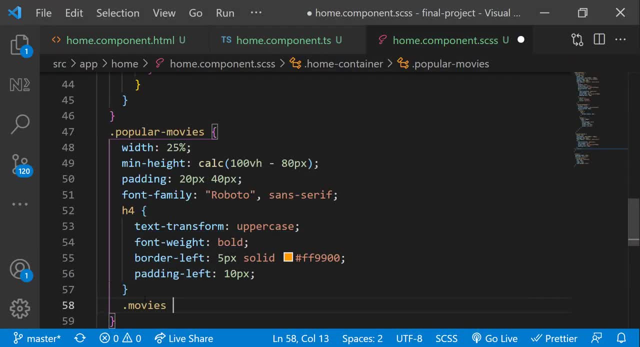 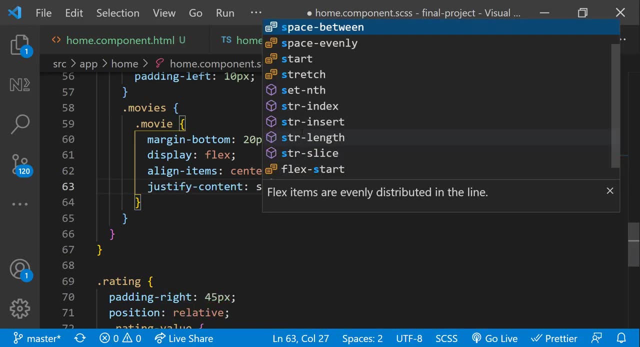 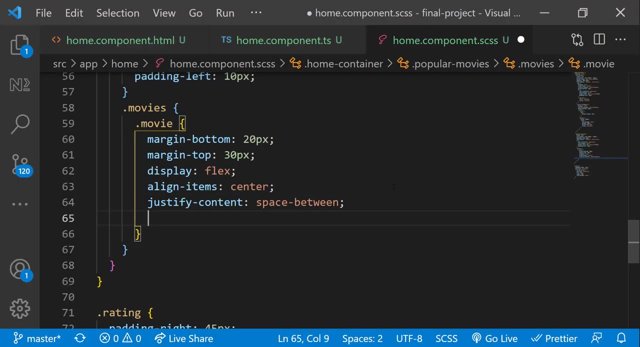 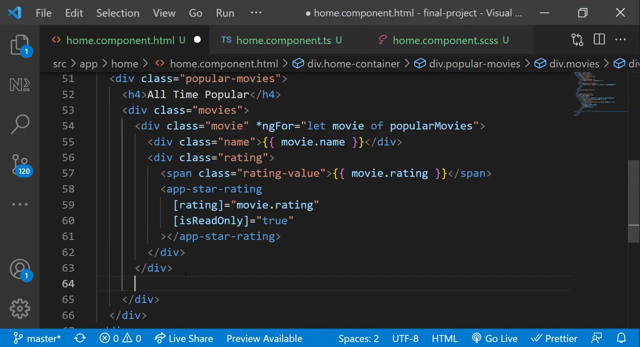 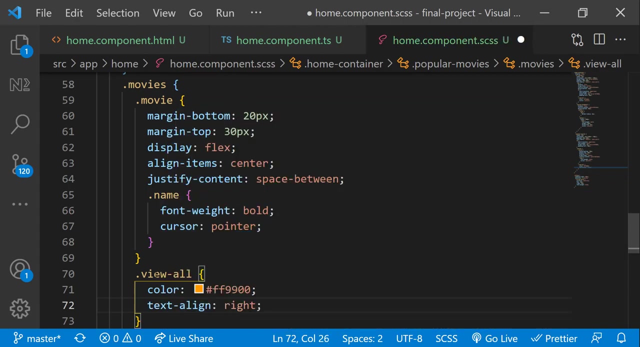 Let me first add a margin bottom here And then apply some styles for movies div. Finally, let me also add a view all button in the bottom And apply some styles. Anyway, I am not going to create any page for this today. 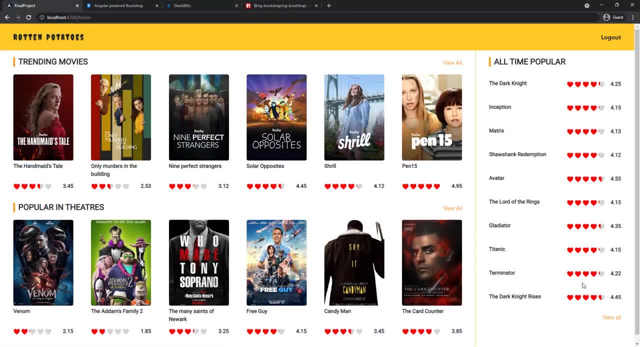 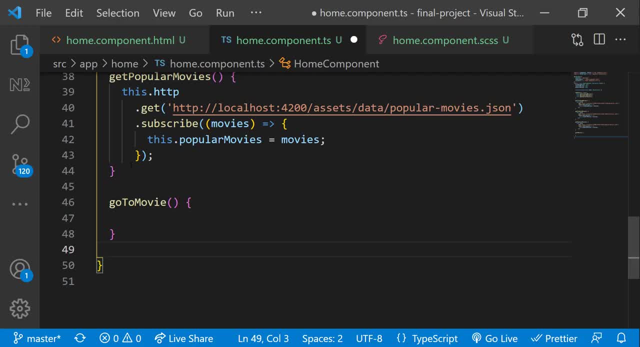 This is just for making the design better. Okay, The homepage looks good. Now I need to add the routing to movie page. For that, let me create a goto movie function which accepts the type of movie and the movie ID as the arguments. 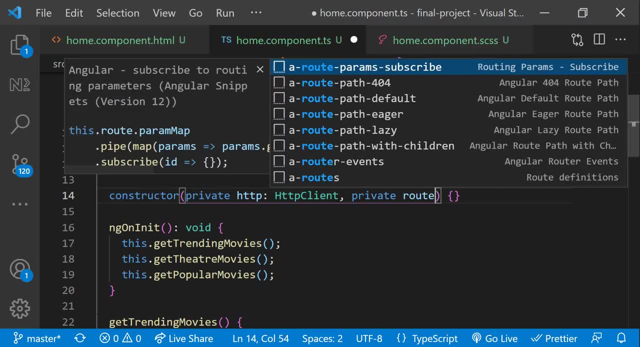 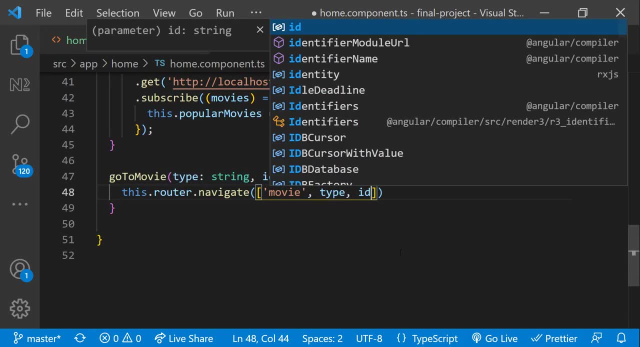 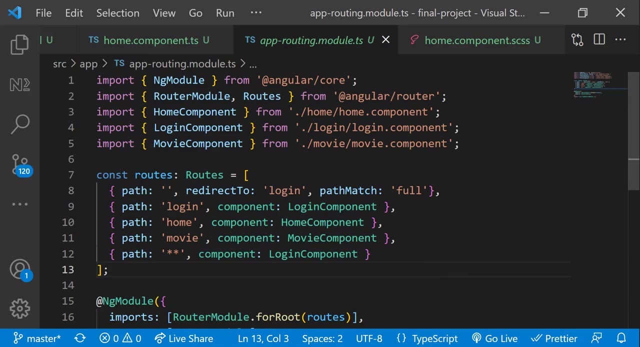 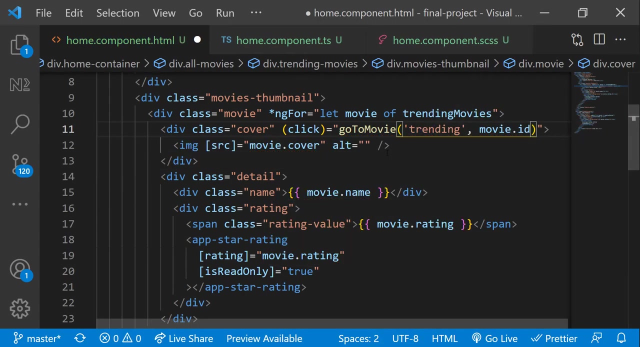 And I can use the router to navigate to movie page. In app routing module I have just mentioned, it has route without parameters. Let me change that first. Okay, In the home html, wherever needed, I can add this clicky one. 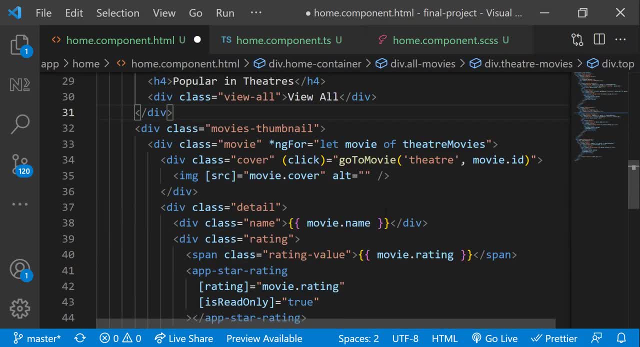 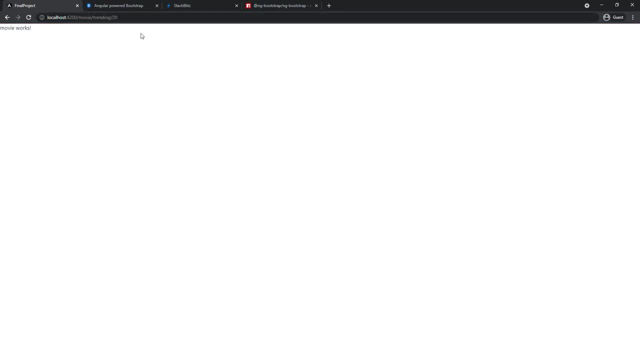 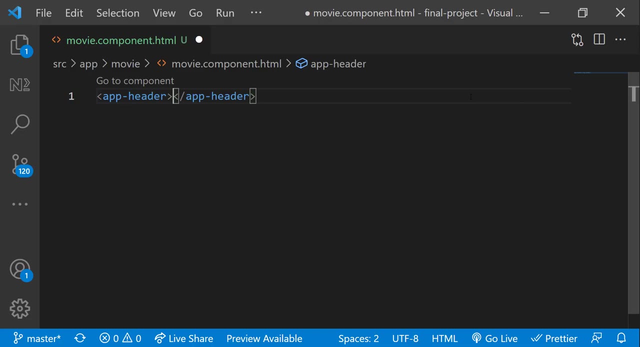 Okay, If I click any, it will take me to the movie page. Now I need to work on the movie page. In movie page, first let me add the app header And then I can add a movie container in which let me create two divs. 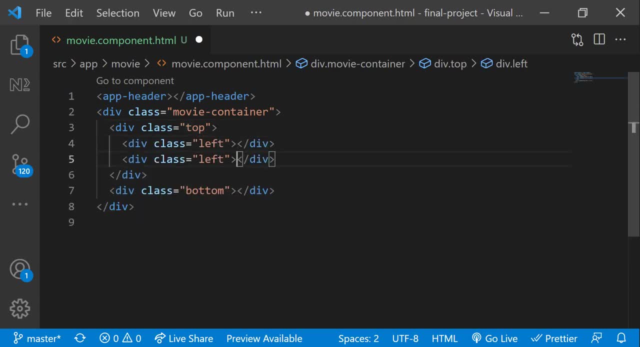 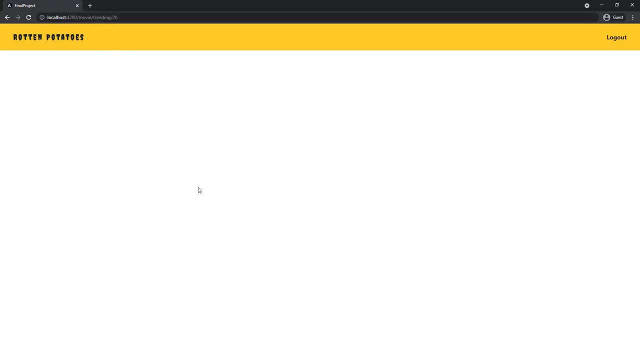 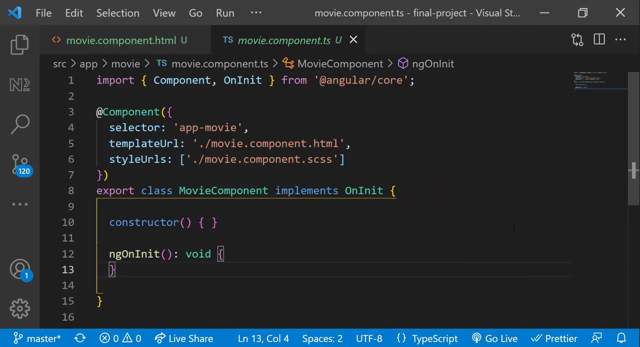 top and bottom. Inside top I am going to create left and right And inside left I want to show name, rating and cover image. Before applying some styles, let me get the movie details First. I need to get these information from the route. For that, let me create two variables. 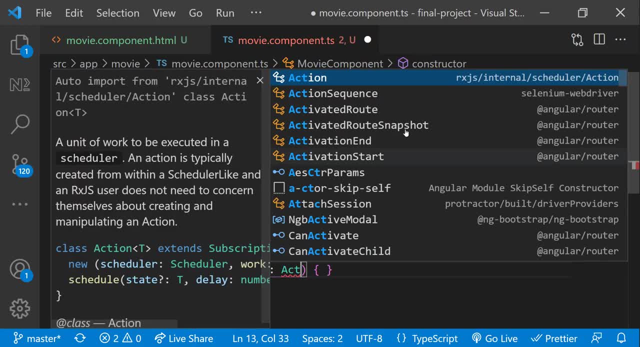 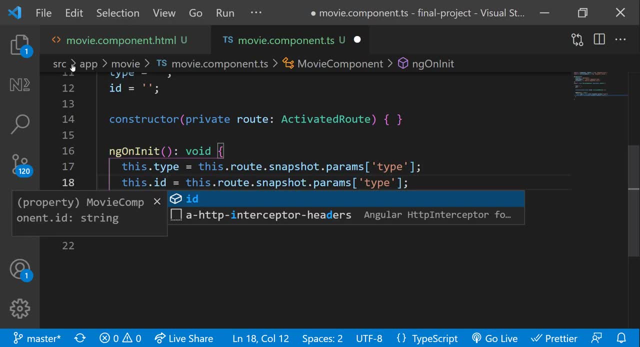 In ngOnInit using the activated route. let me take these params from the route snapshot To get the movie details. let me create one function and call that in ngOnInit, Inside the function, using http client, I can get the movie information. For that, let me create. 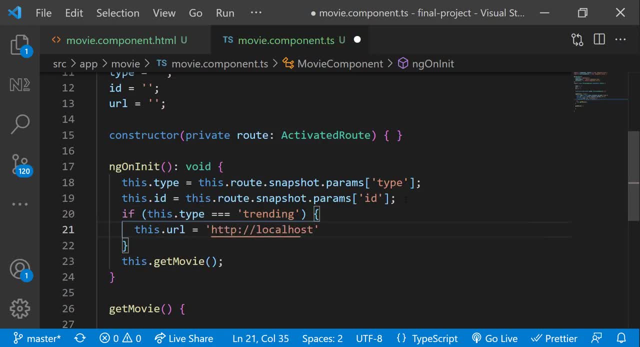 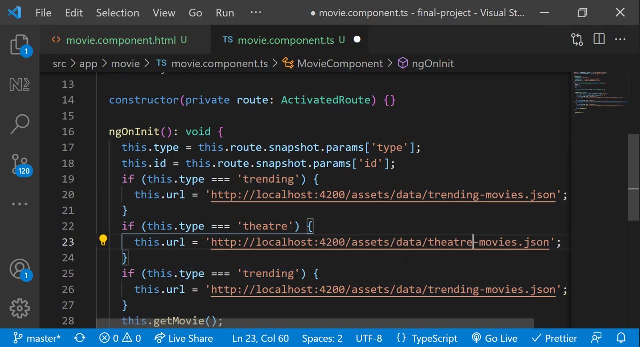 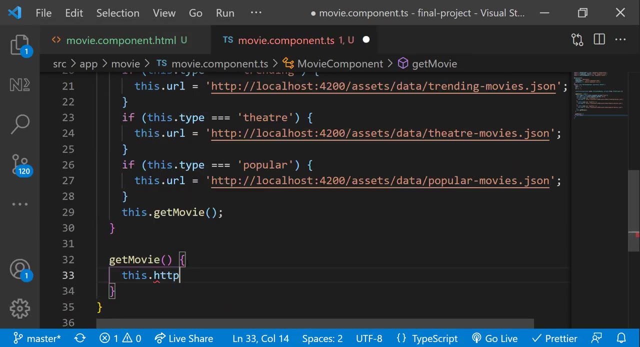 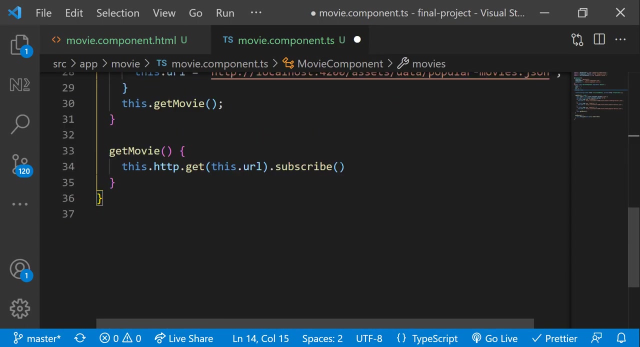 a variable called url. And in ngOnInit, based on the type, let me assign the right value to the url. And in getMovie function, let me pass this url and subscribe to get the response. Let me create a variable to store this response. 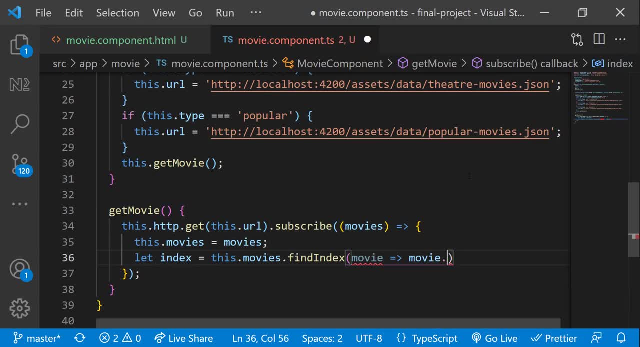 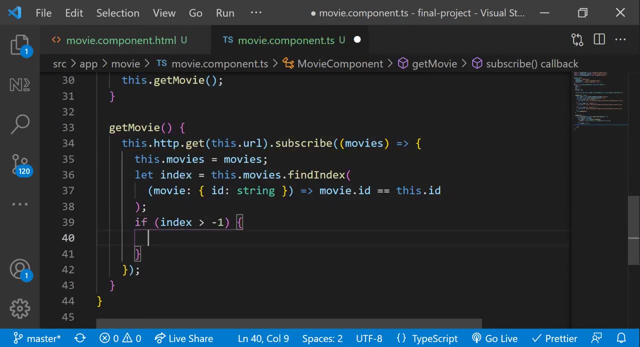 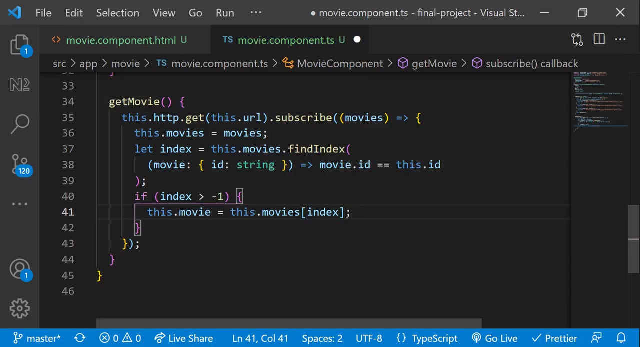 And using the findIndex method I can find the position of the movie in which the id is getting matched. And if the index is greater than minus 1, then I am assigning that movie in a variable. So now we got the movie information in this variable. 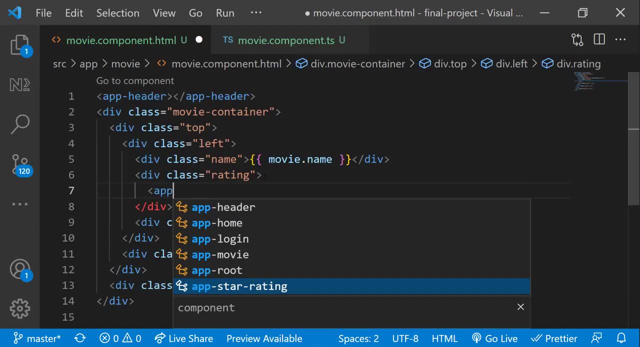 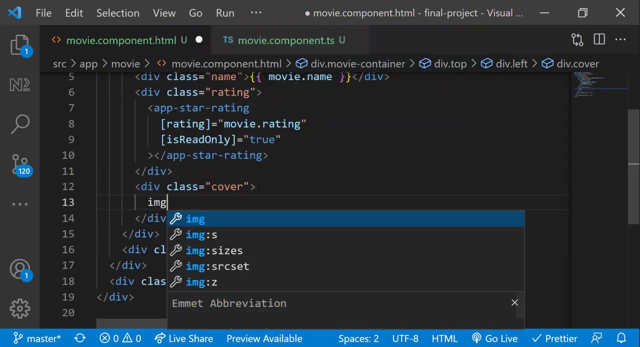 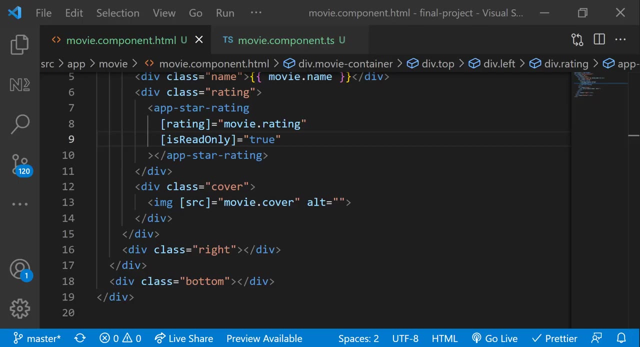 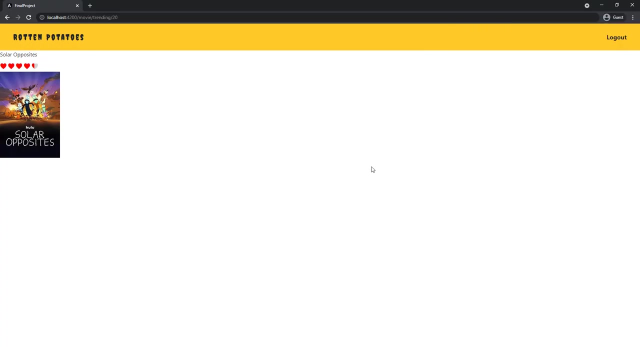 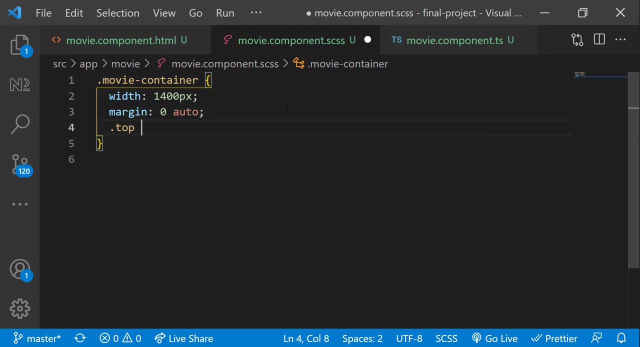 Let me go back to the html and bind the right values. Okay, Now, if I preview, we can see this. Let me apply some styles. First, let me bring this container to the center, And for the top let me use display-flux Inside top. for the left, let me give 450 pixels. 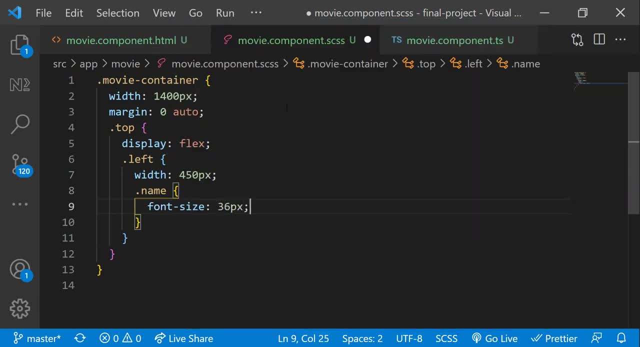 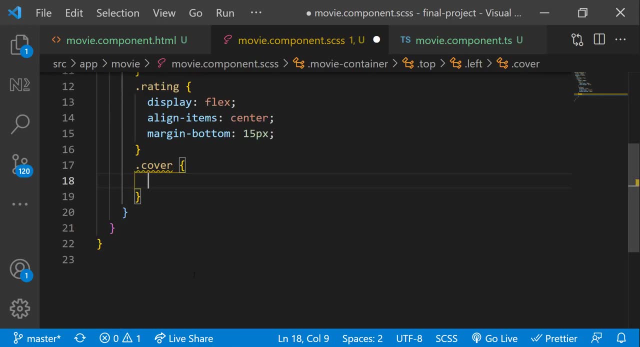 And for the name, let me use a font-size of 36 pixels and bold. For rating, I am using display-flux, align-items-center and margin-bottom of 15 pixels. And for cover, let me give width 400 pixels and height 500 pixels And margin-right 50 pixels. Inside that for the image width. 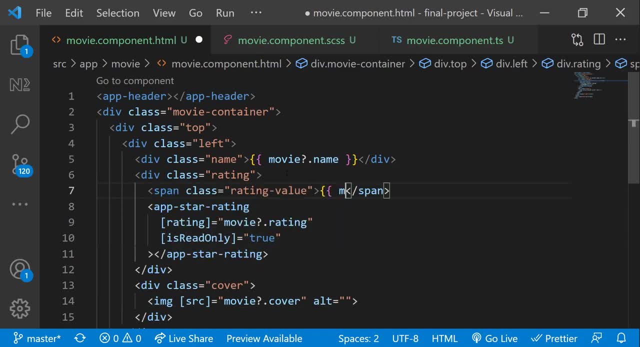 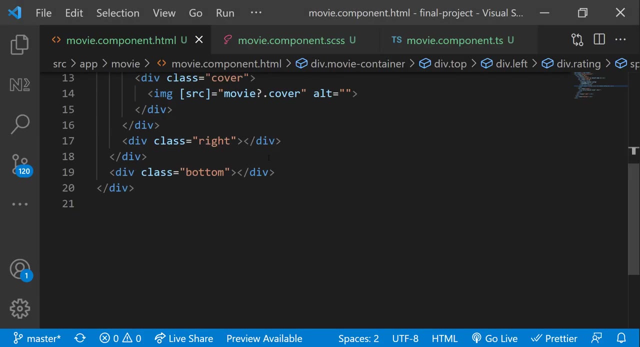 100%. height, 100% and object-fit cover. And for the rating value, let me give margin-left 20 pixels and font- suspension-wide 8.. Okay, It looks good Inside the right div. let me create a form so that the users can submit their review. 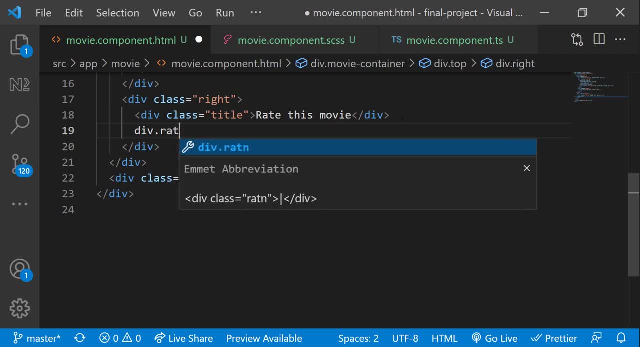 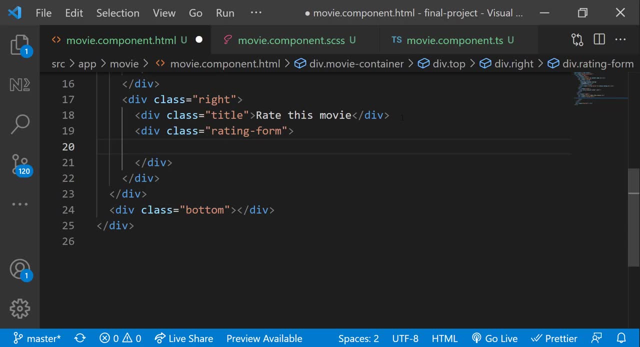 Let me add a title first and then a div for the form. I need to create a form group for getting the user's name and then one rating field so that the user can rate and one text area for getting the review content. 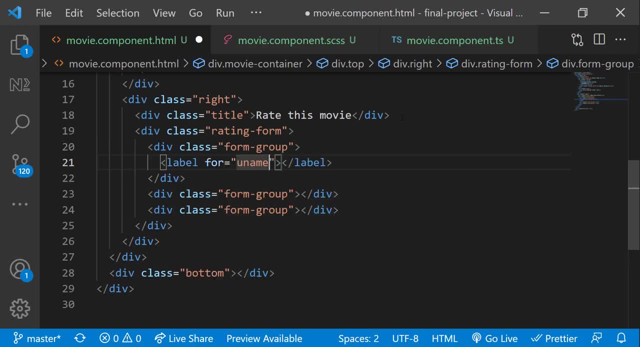 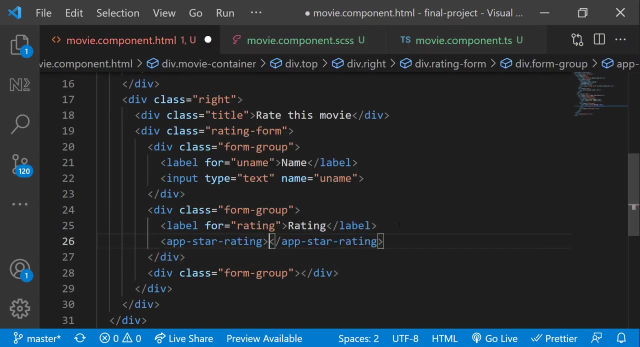 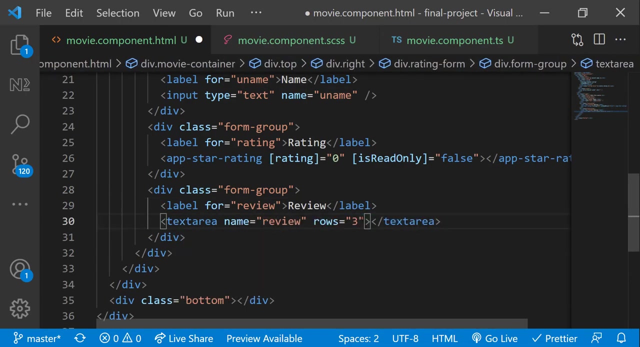 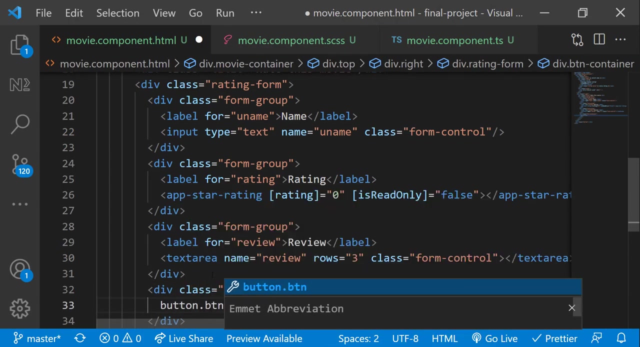 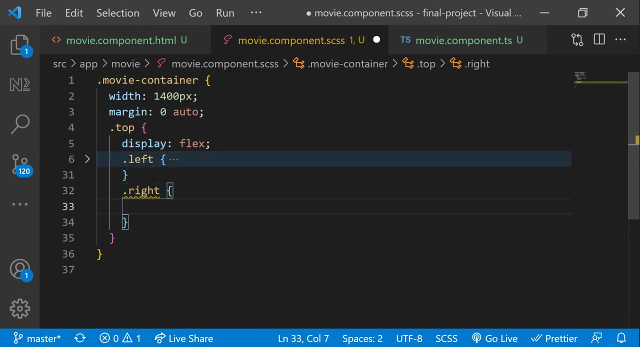 Thanks. So three form groups: first one for username, second one for rating, in which I can give, if read, only false this time, and the last one for getting the review. Finally, we need to have a button. Let me apply some styles. 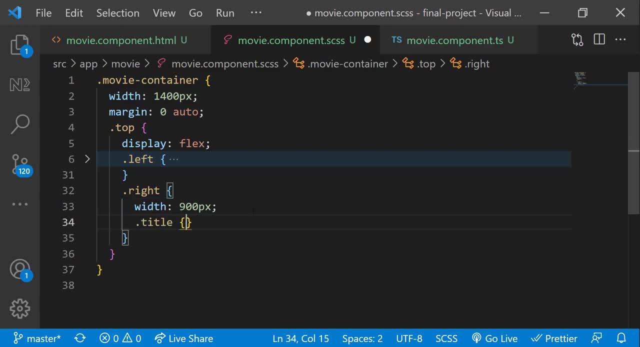 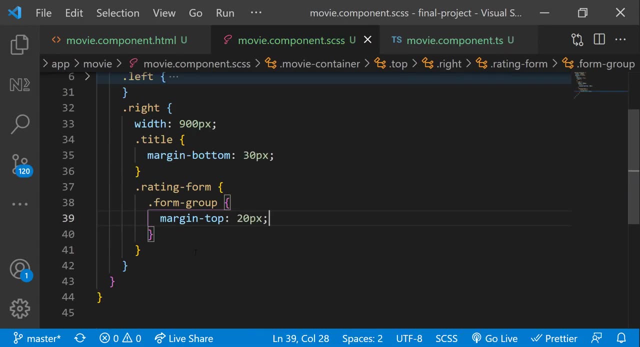 For the right div, I can use a width of 900px, and for title, let me give a margin bottom, And for form group, let me give a margin top- 20px. let me add a padding top so that this comes down. 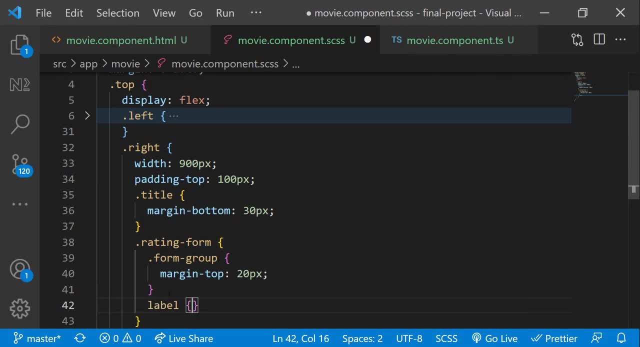 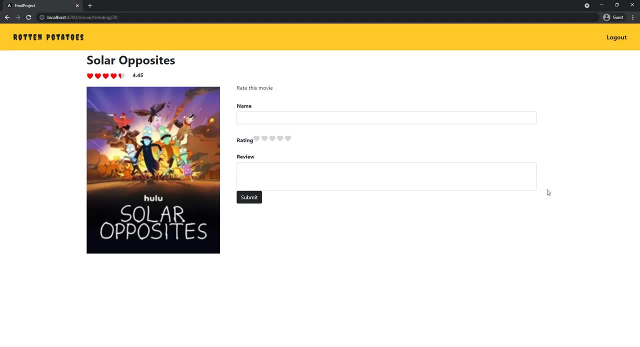 And for the label, let me give font-weight, bold and margin bottom: 5px. Okay, and for the text area, let me apply resize: none. Now let me bring this down. Okay, looks good. Now let me show the reviews in the bottom. 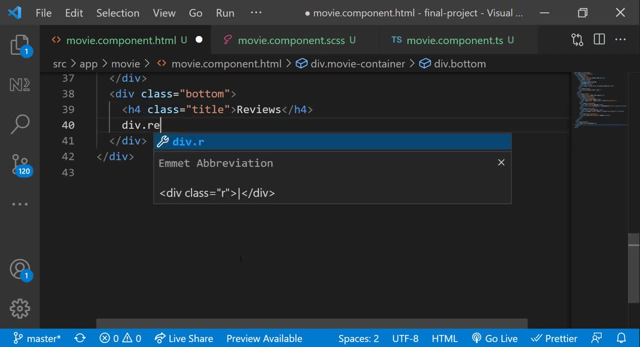 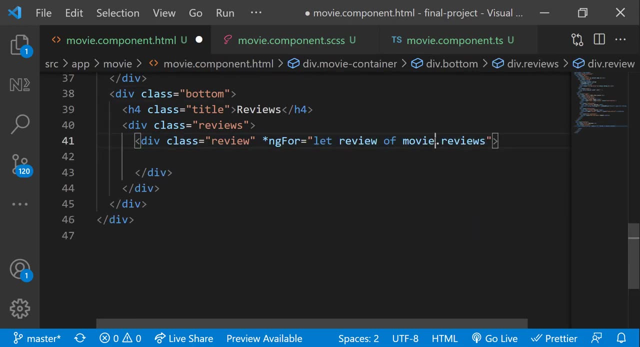 I'm going to add a title and then a div to hold all the reviews Inside that. let me use ng-reviews- ng-for to show all the reviews one by one Inside review div. let me create review details and then review text. 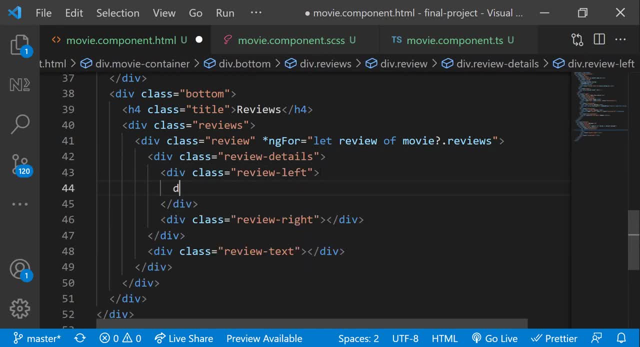 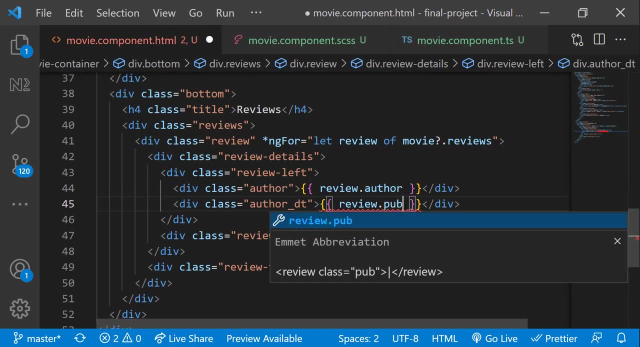 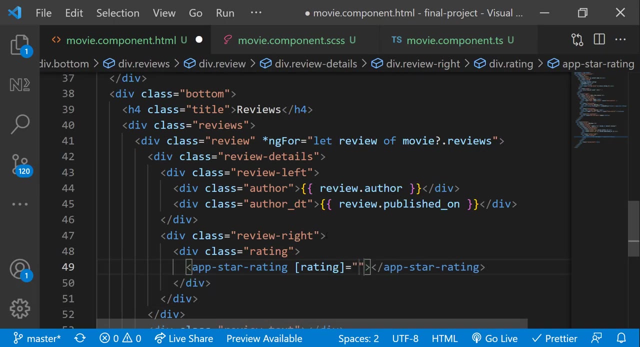 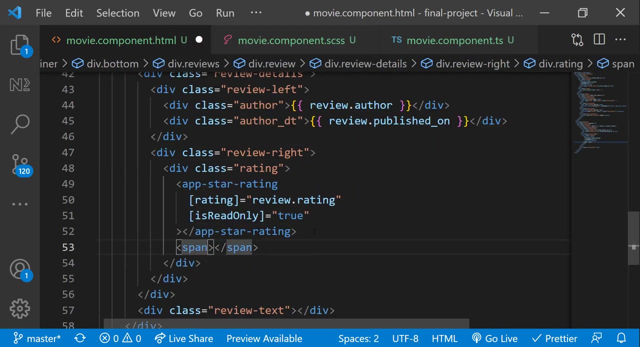 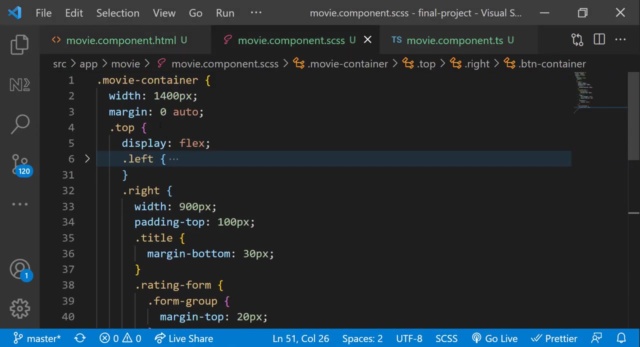 In review details, let me create review left and review right. In review left, I can have author name and the published date, And in review right, let me have the rating. Okay, it's showing like this. I need to apply some styles. 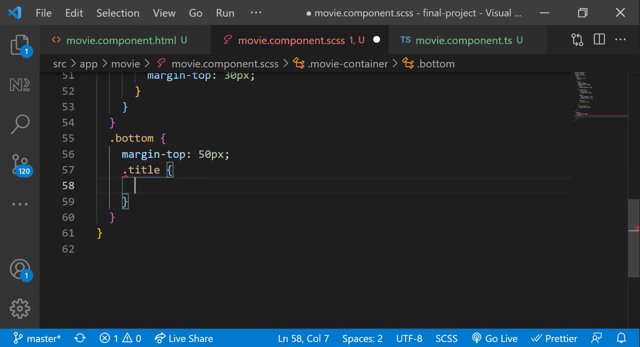 First, for the bottom div, let me apply a margin top of 50px, and then for the title, a margin bottom of 30px. and then for reviews div, let me give a width of 1000px. For each review, let me add some margin bottom and a background color, also a padding, and 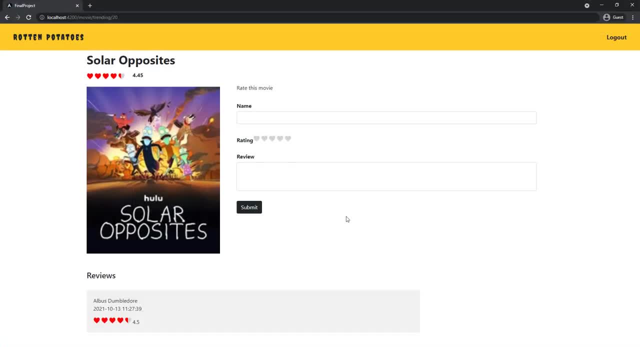 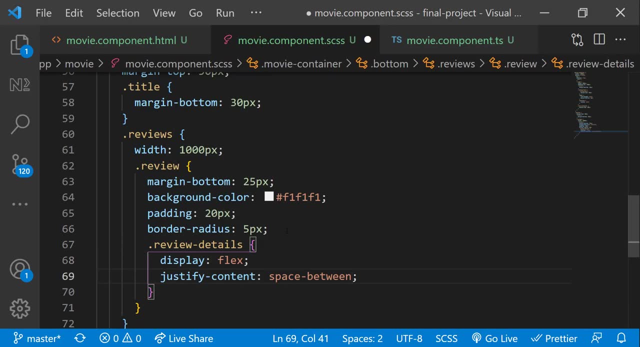 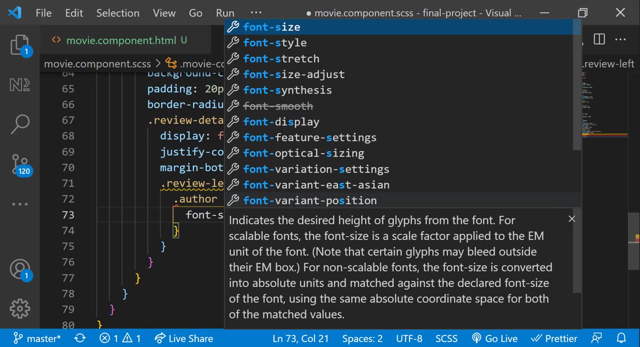 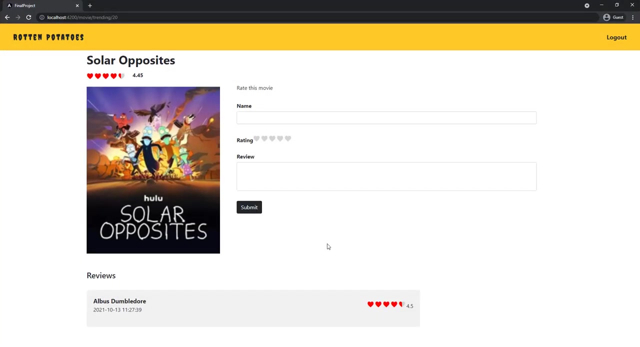 border radius of 5px. Okay, For the review details, let me give display flex: justify content. space between and margin bottom: 20px. For author, let me give a font size of 18px and font weight bold. And for author date let me give opacity 0.7, and so it appears little lighter than the. 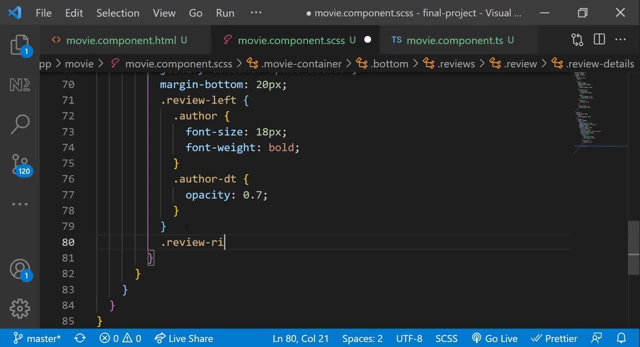 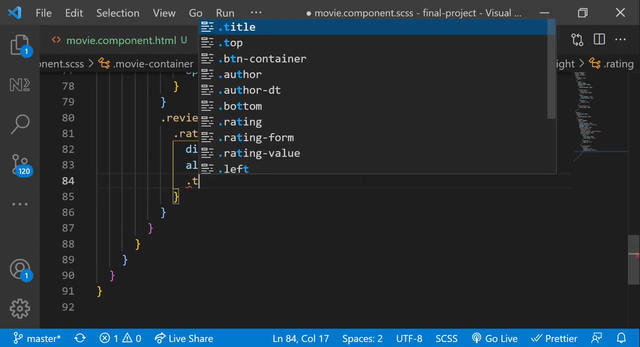 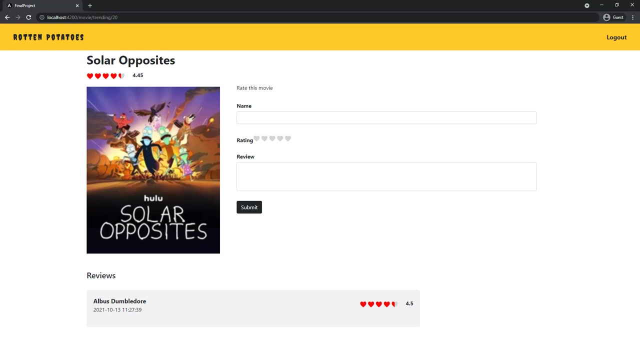 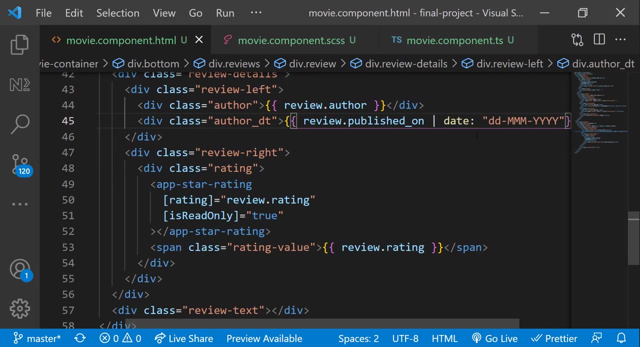 name. For rating, let me give display flex And align item center, And for rating value, let me give margin left 20px and font weight bold. Okay, this looks good. Let me also format this date using date pipe, And for some movies there may not be any reviews. 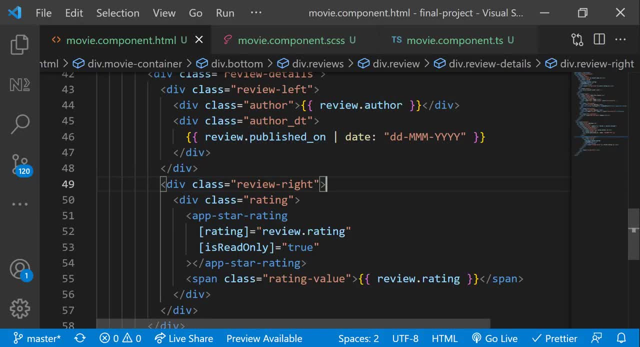 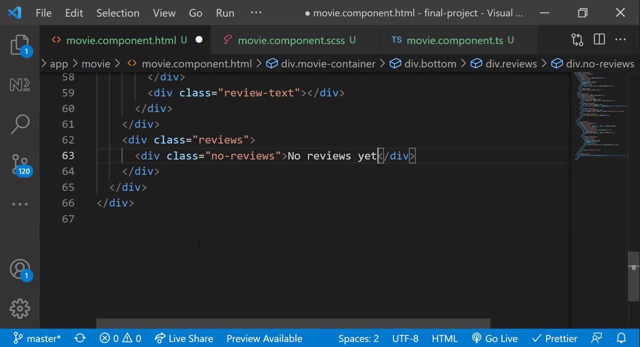 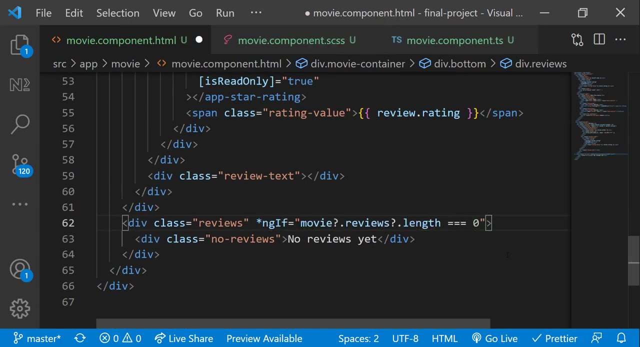 Let me also handle that. So let me create another div for showing a message- No reviews. And when there are reviews, let me show the first div, And when there are no reviews, let me show the second div. Okay, let me test it completely once. 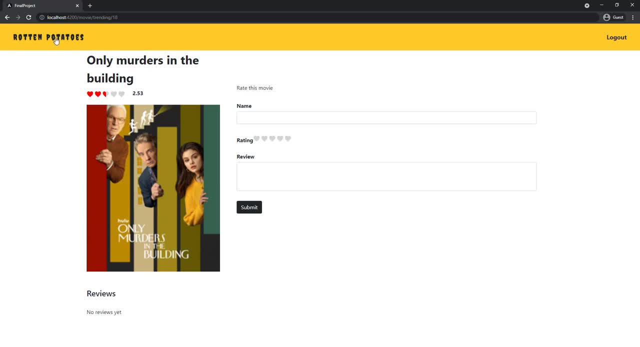 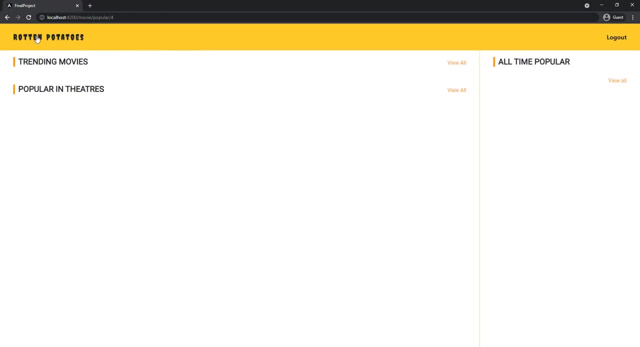 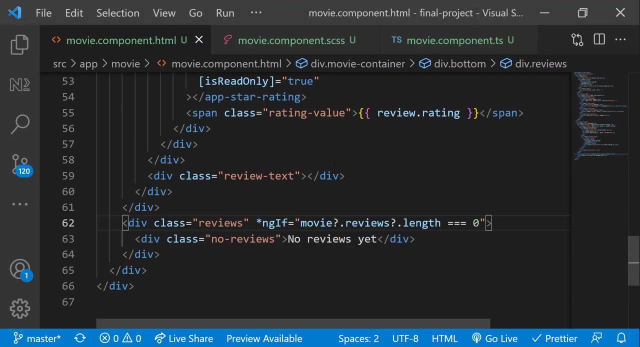 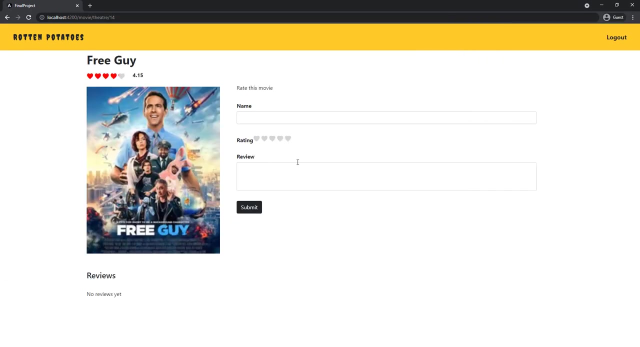 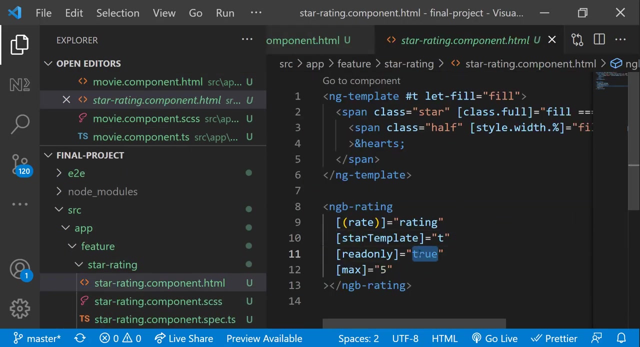 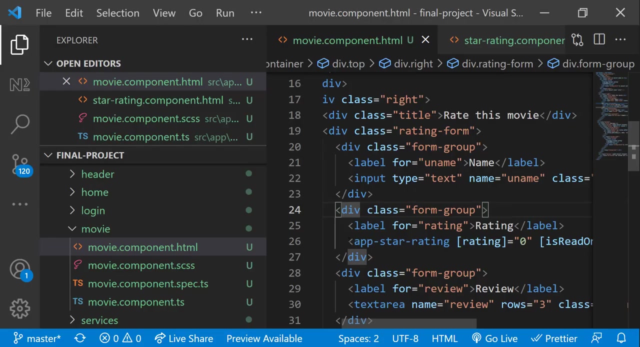 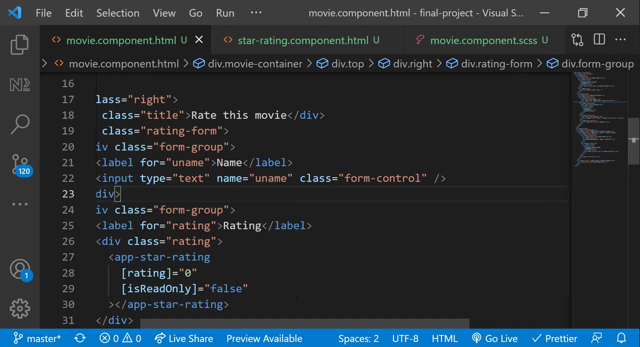 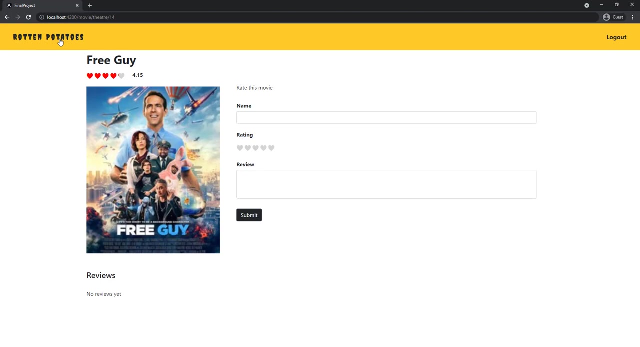 Okay, this is fine. Okay, I can go back you. I think this is working as expected. as I don't have a database now, I'm not going to handle this form functionality, but I believe this is almost a complete application through which you can.